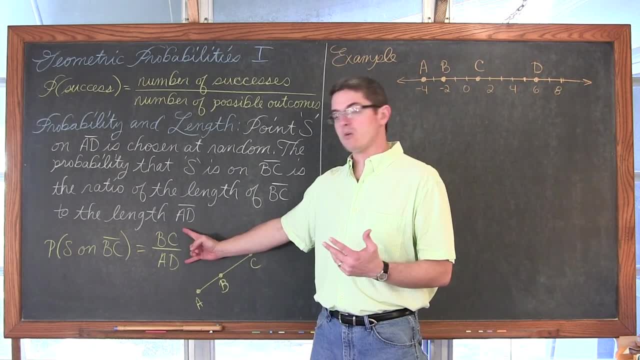 of AD. And again, remember, when you are talking about lengths of segments, you don't have the sort of segment line on top of that. This is segment BC, this is length BC. so we are going to find the length of BC and 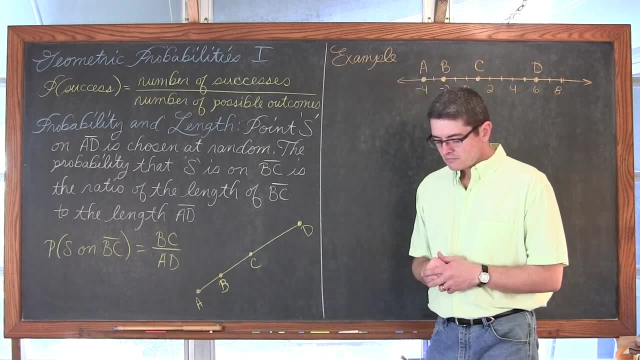 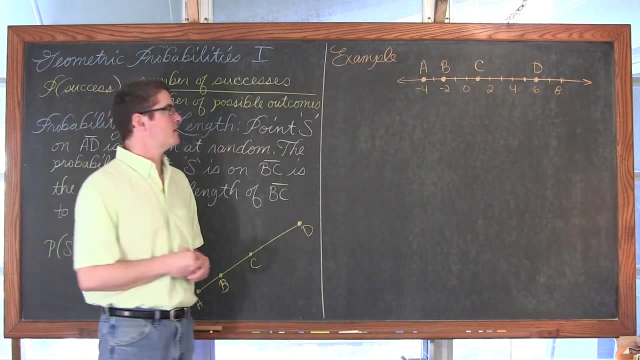 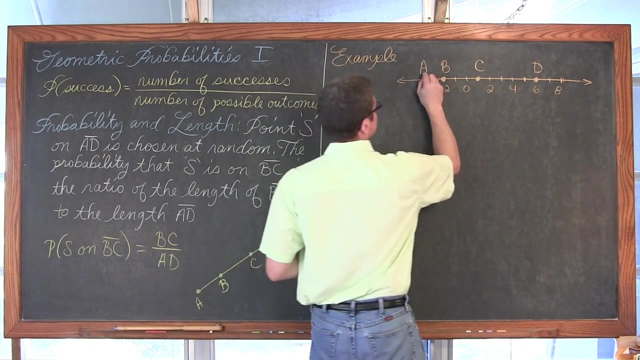 divide it by the overall length of AD. Ok, so let's take a look at our two examples. The first one is going to be a very simple example. We just have some values on a number line, So I have placed a number line, but we are talking about segment AB, excuse me, segment. 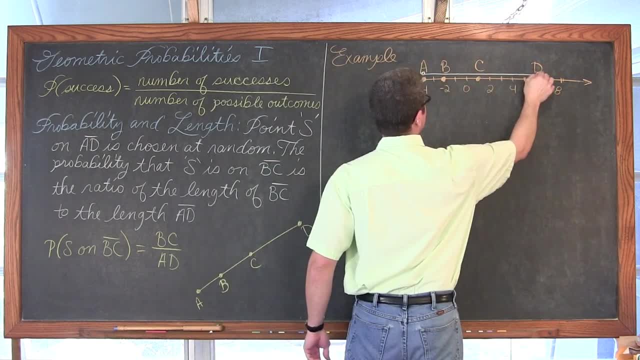 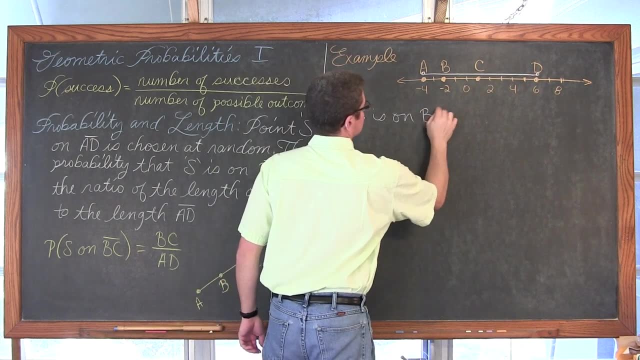 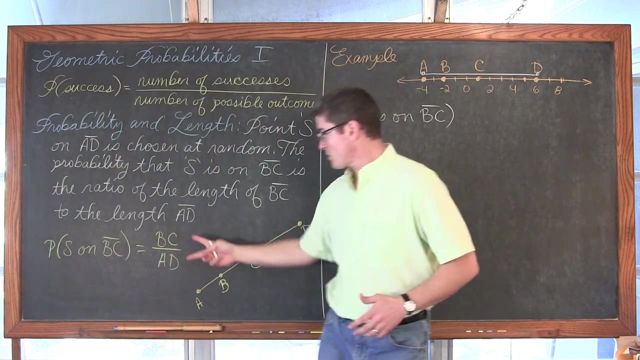 AD. So I want to find the probability that S is on BC. Now, length on a number line, since that is what we are doing, length on a number line is pretty easy to calculate. You really just can kind of count along the places. 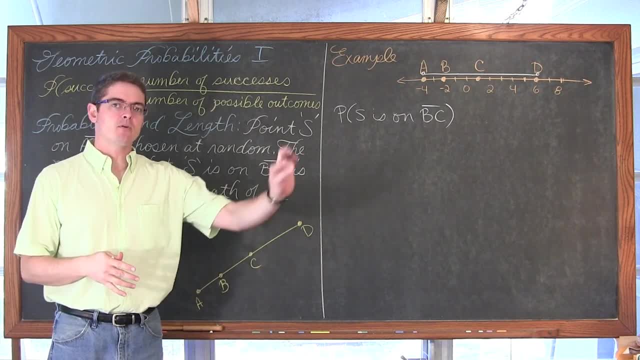 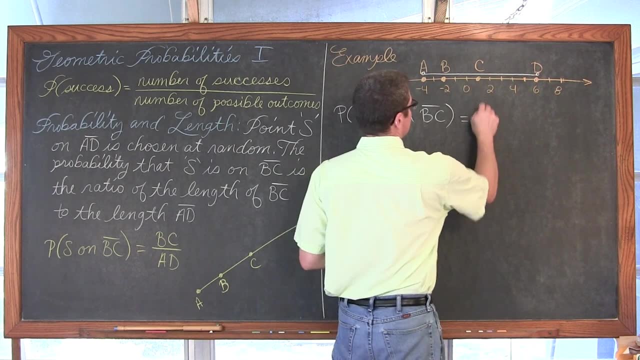 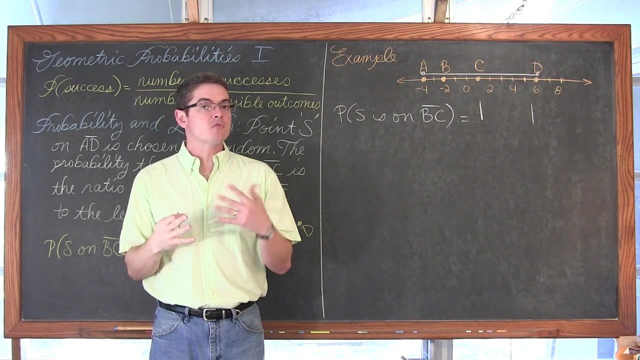 But if the numbers are a little bit weird and you can't just simply count your way from the left point to the right point, Then the distance on a number line is going to be equal to the absolute value. we are going to take the two numerical values along the number line we are going to subtract. 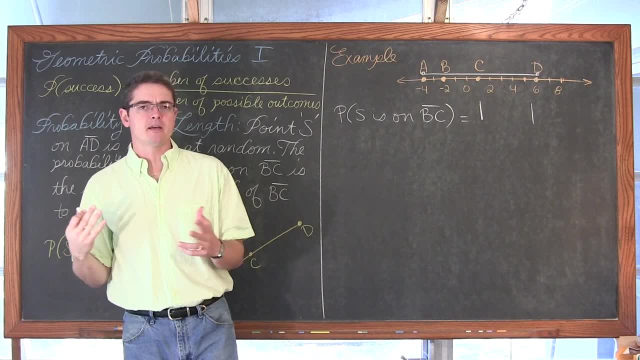 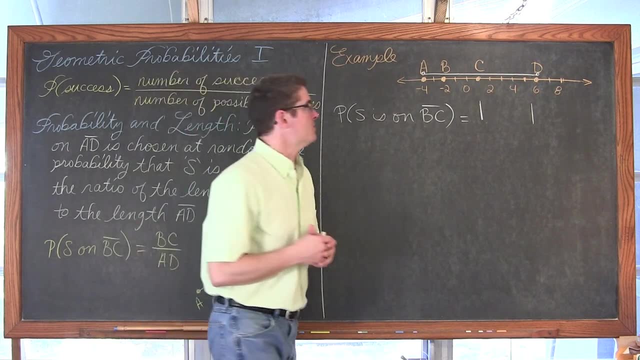 them and take the absolute value of that, Because you can't have a negative distance, like you can't have negative distance, you can't have negative length, negative area, negative weight, You can't really have negative measurement values. So I am going to pick. I want to find the length of BC. 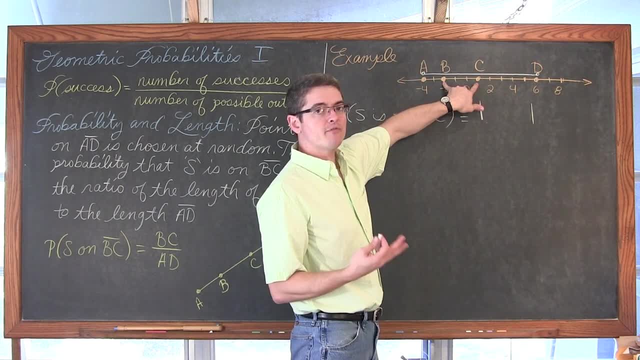 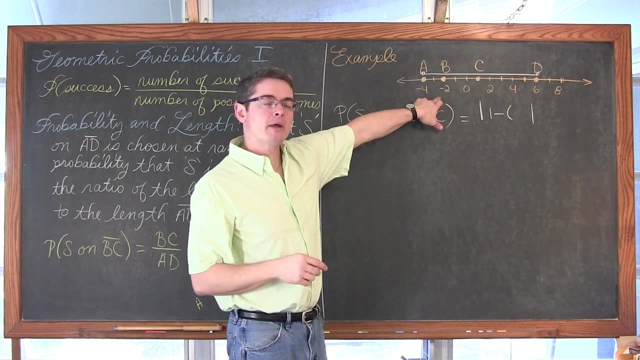 And so here is B at negative two and C at positive one. So if I want to find the length of this segment, I am going to take the value of one for C, I am going to subtract that with the value of B, which we have, and point B is placed. 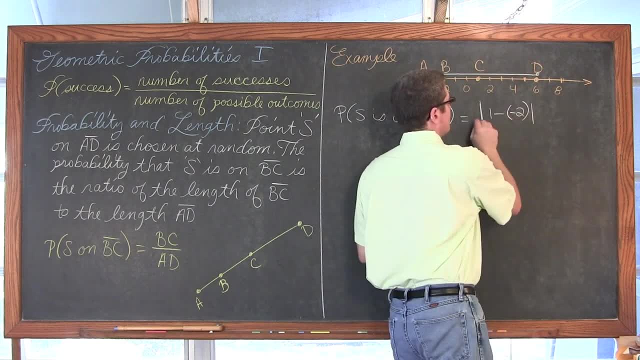 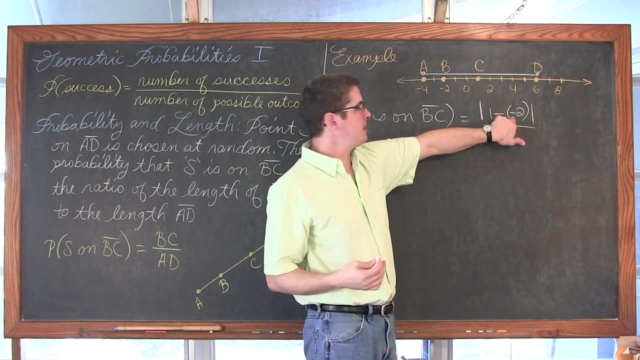 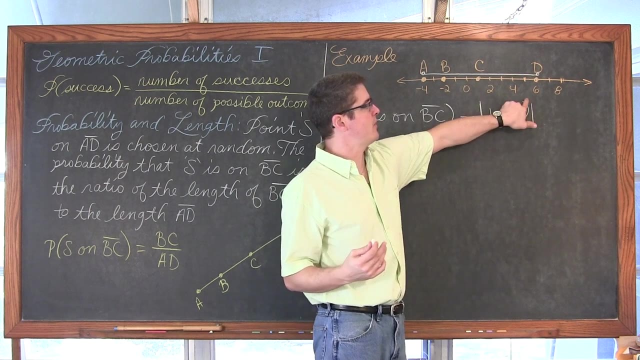 on the number line at negative two And I am going to subtract that. well, I am going to work this way down. When you subtract a negative, it is really like negative one times negative two, which is addition. So when you have two negatives right next to each other, like this, and there is no exponents, 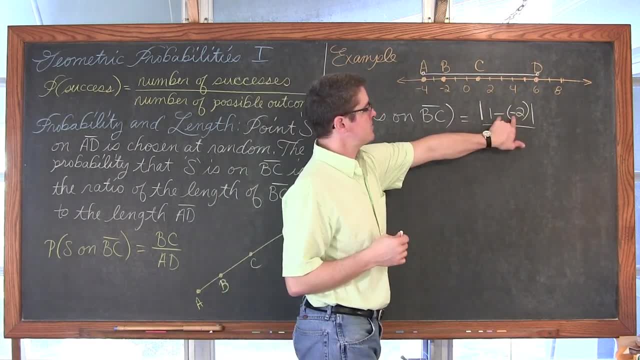 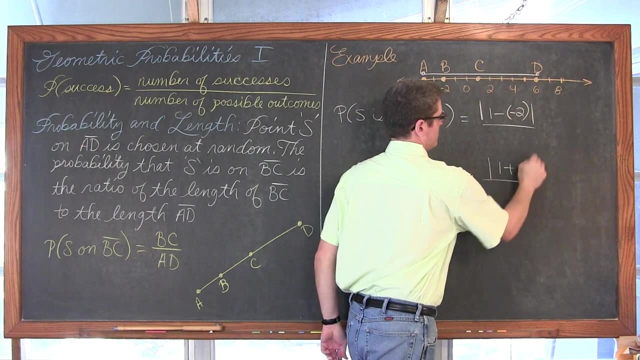 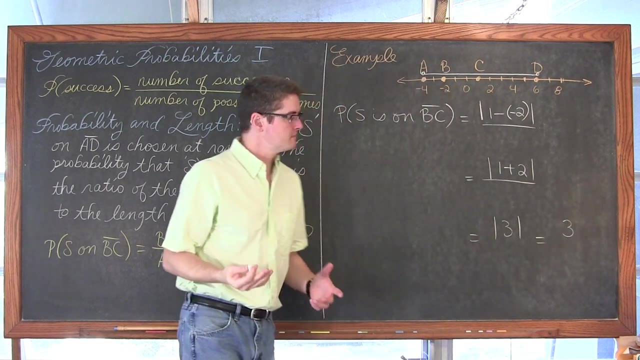 or other mathematical steps you have to do. first, Those two negatives cancel out to be a positive. So that is going to be the absolute value of one plus two, which is going to be equal to the absolute value of three. Well, the absolute value of three is just three. 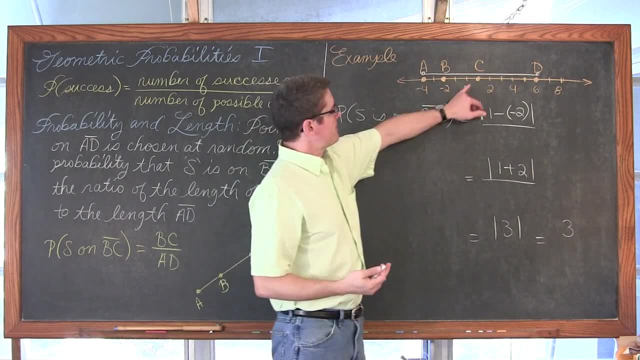 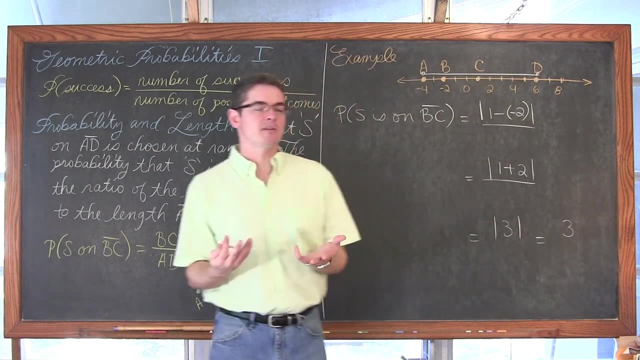 Well, ok, I am doing the top separately because I set it up. I did basically the large number minus the small one, So I was going to get a positive distance, And so thus the absolute value symbol didn't really do anything. Now, by the way, an absolute value function tells you how far a number is, how far a numerical. 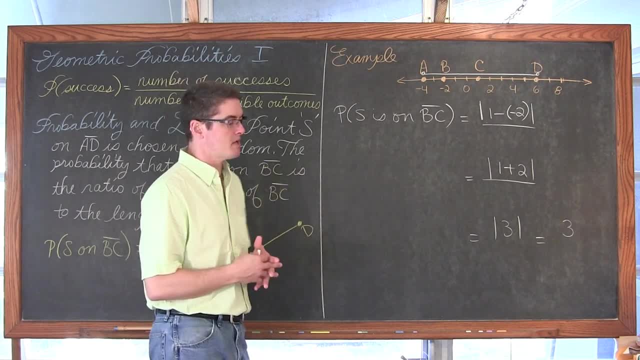 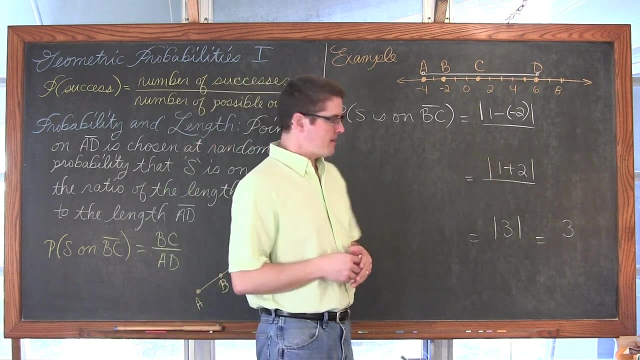 value is from zero on a number line. That is really what the absolute value symbol does. We often just think of it as eh, it gets rid of the negative sign. So let's say again the importance of the absolute value sign and why we have to include. 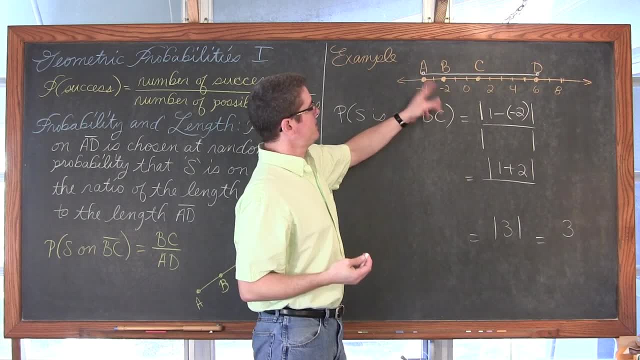 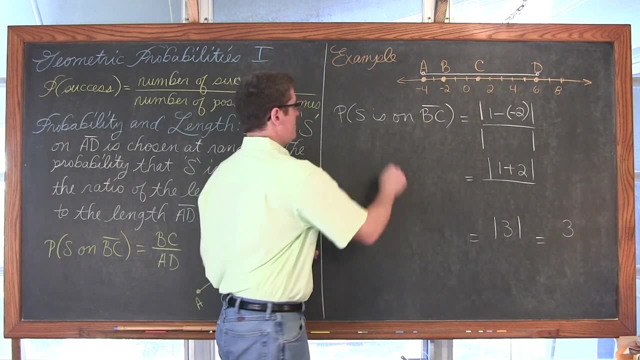 it when we find the distance along the number line is maybe for finding the overall length of AD. so it is again part over whole. the probability that S is on BC is going to be the length of BC. The length of BC over the length of AD is well, let's just say here, let's just take 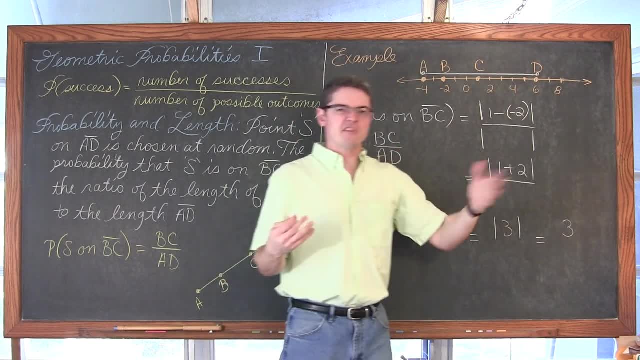 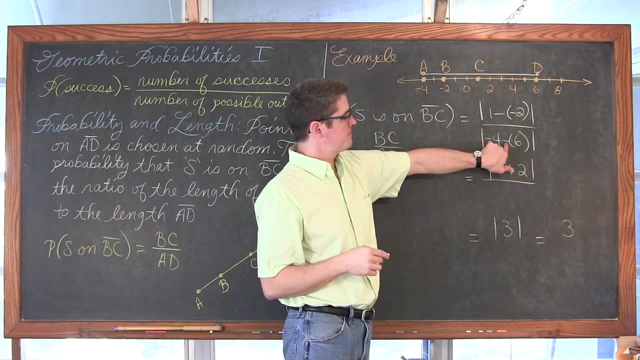 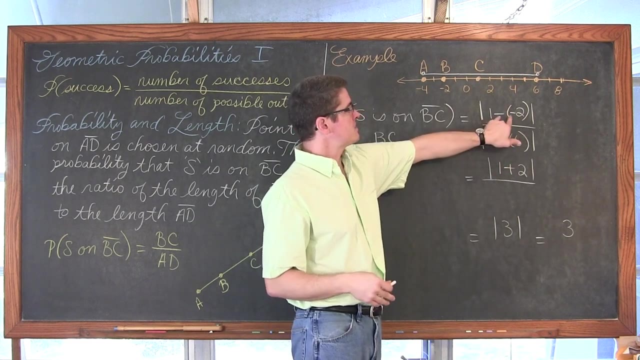 the negative four and subtract it with the six. So I am reading it like left to right And we get negative four minus six, and we are. I always have a habit of using parenthesis when I subtract or, excuse me, when I substitute, and that is so that if there is a minus in 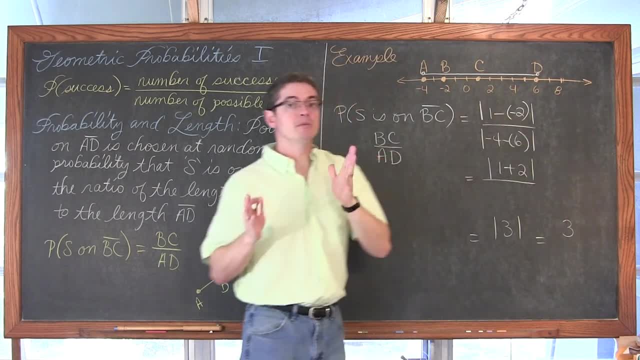 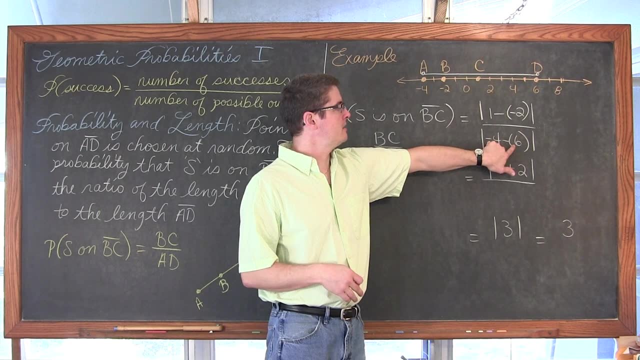 my formula and a negative from the value I am plugging in. I remember to write both and if they need to cancel out They will. So four minus you know you could write four minus six. I always use again parenthesis. 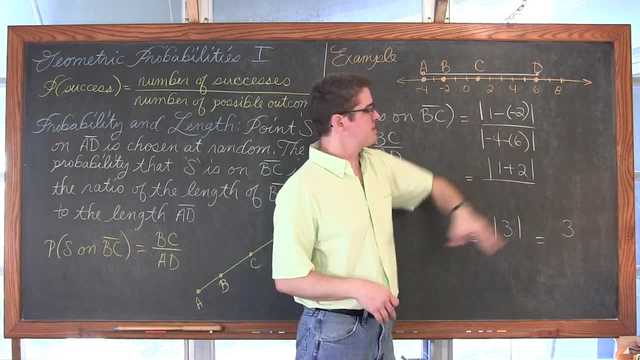 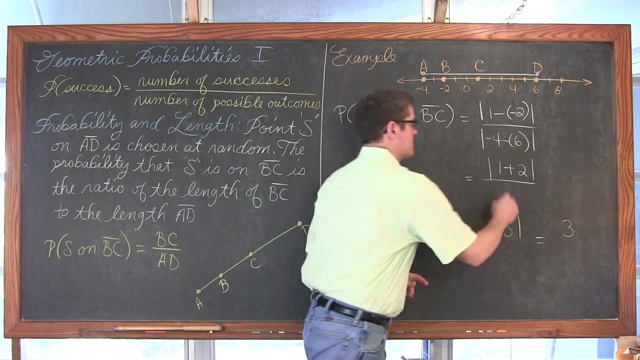 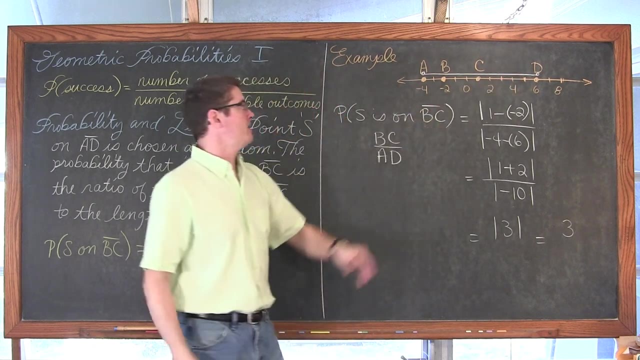 when I do substitution though. So I have negative four minus a positive six. So negative four minus six. when you combine numbers with the same sign, you add those numbers and keep the sign. So negative four minus six is negative ten. Now see the way I have picked my two values, or used my two values of where is A and D? 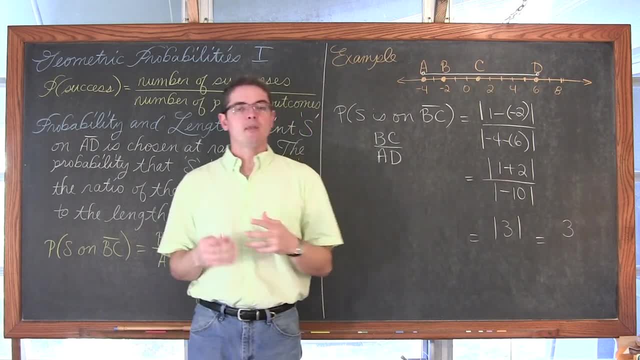 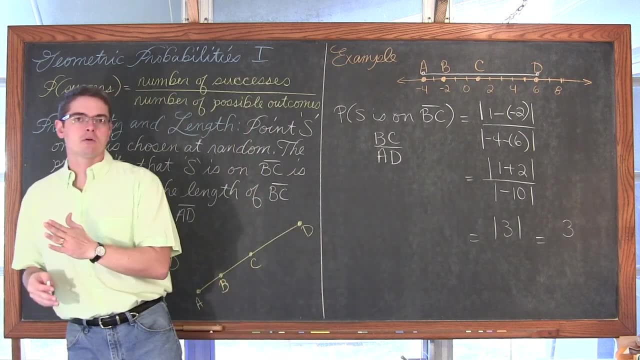 on the number line, I have ended up with a distance which is negative, But as a measurement That doesn't make any sense. Sometimes in geometry you do have like negative numbers, but maybe they indicate moving backwards or negative rotations as opposed to a positive rotation. 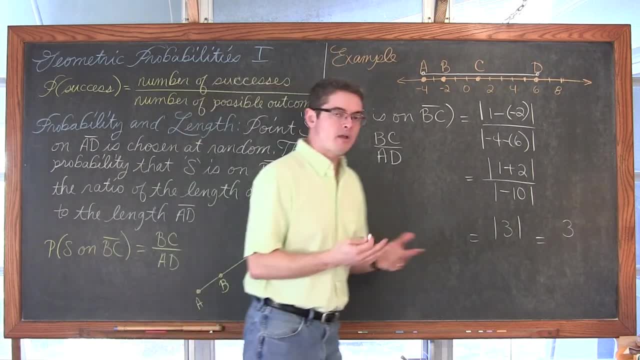 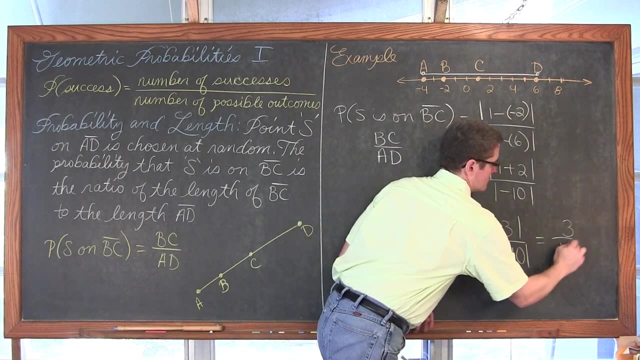 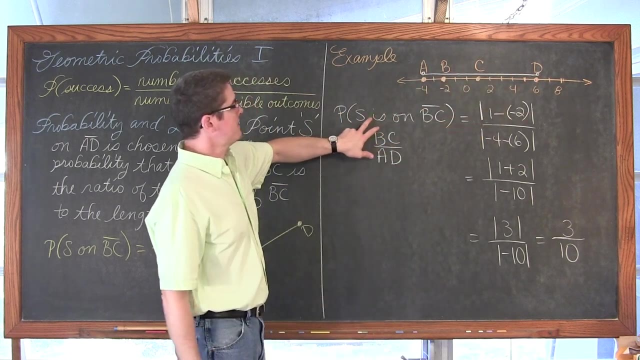 But as a pure measurement of length, area, volume and such, you can't have that. it can't be negative. So the absolute value of negative ten is positive ten and the probability if I randomly choose a point along this segment of A- D, the probability that a randomly chosen point is positive ten. 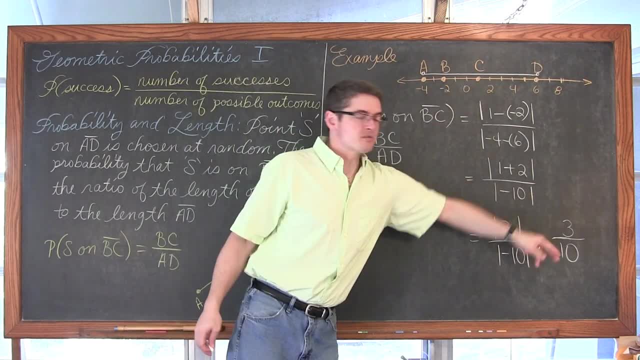 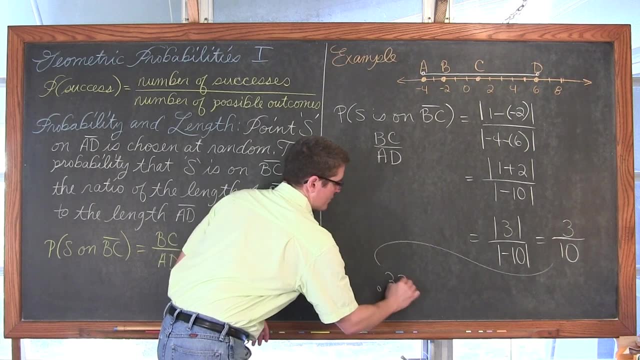 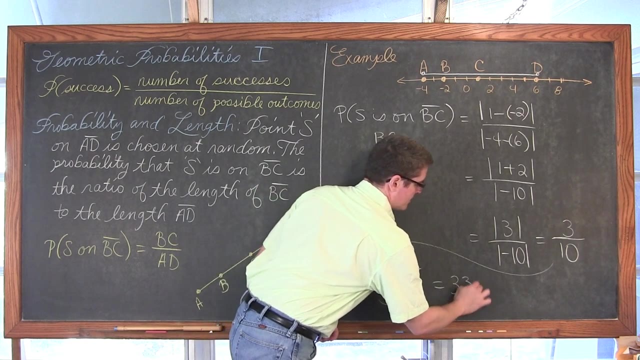 is positive ten. So my probability on just this part of BC is three tenths. So my probability is three tenths. Or you can write that as a decimal, as .33, and that's going to repeat, which would be equivalent to moving that decimal over two places and saying that it was 33.3%. 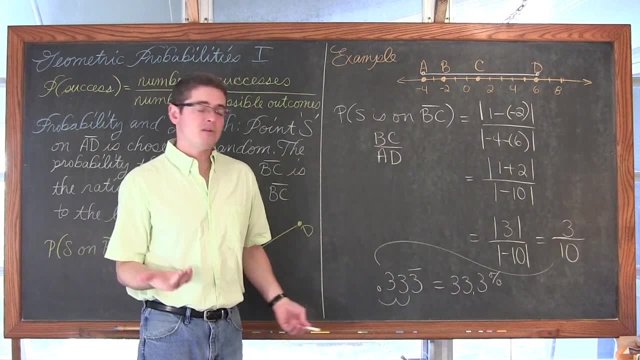 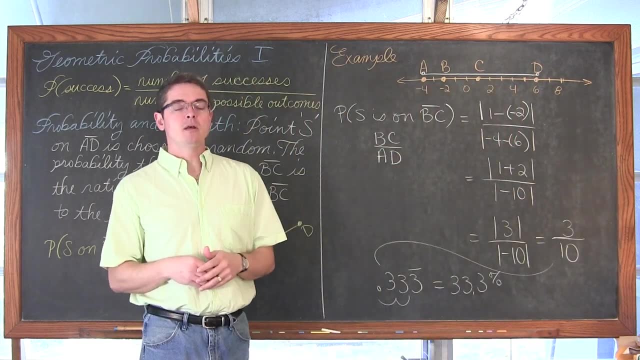 You're just going to write your answer. however, your teacher wants you to do so. I've got one more example involving length. that's not going to be on a simple number line, So we will be using it. I'm reminding you how to do it. 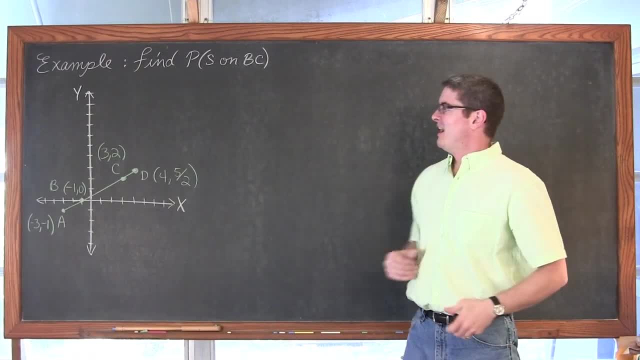 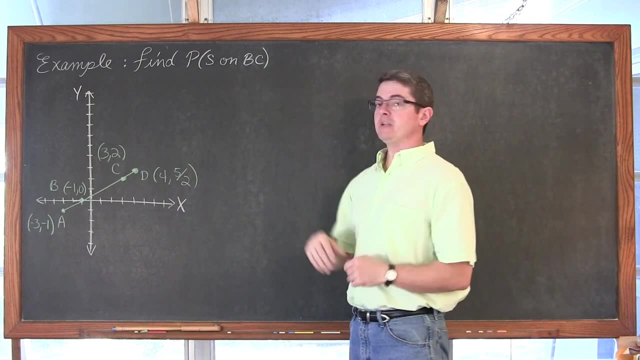 We're going to do the distance formula, All right. Last example: I've got a line segment. again It is at an angle, so we can practice the distance formula which says: find the probability again that S is on segment BC. You don't necessarily have to find the probability that a segment is just on this piece. 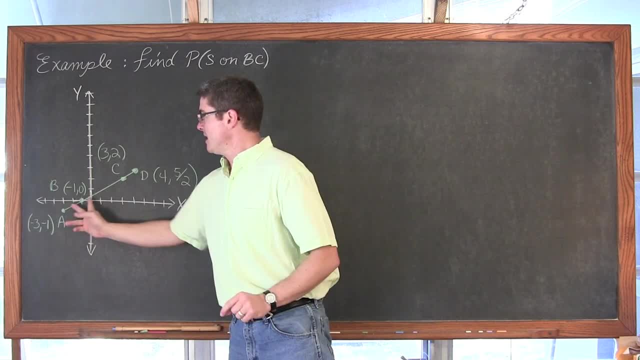 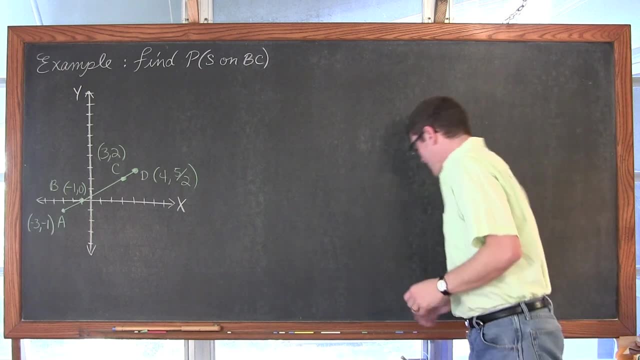 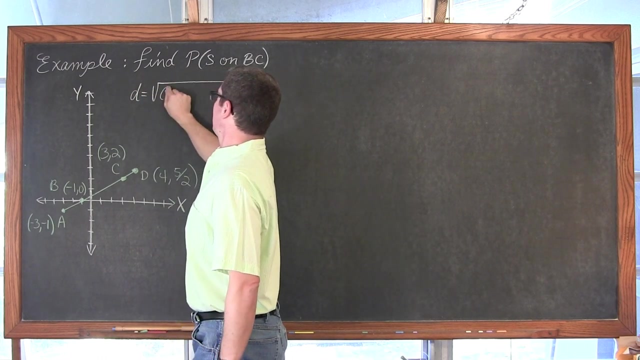 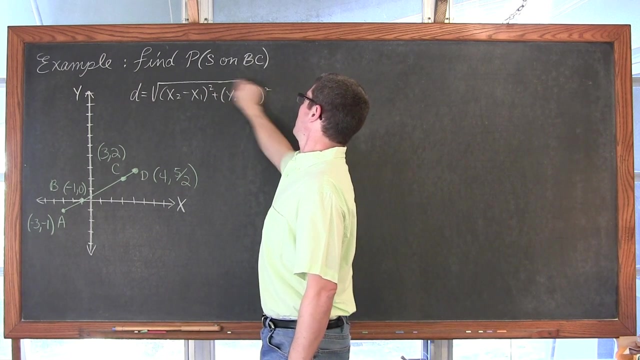 I can find the probability that the segment or the randomly chosen point is on AB or BC or CD, for that matter. I'm justwhatever, It's just what I set up. And Well, your distance formula is the square root of x-sub-2-x-sub-1-squared plus y-sub-2-y-1-squared. 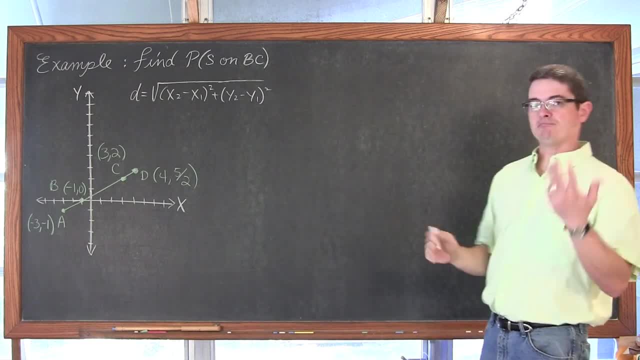 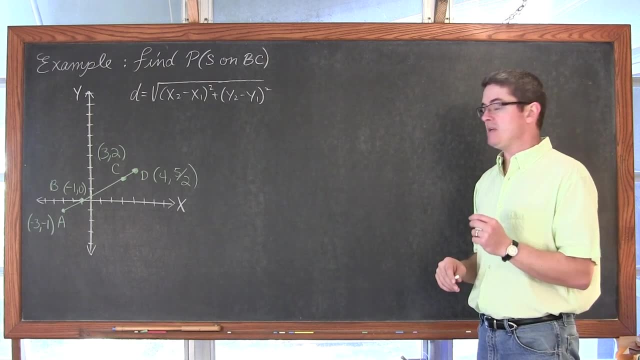 which, by the way, the distance formula is derived from the Pythagorean Theorem, in case you care to know that. And okay, so that means that if we want to find the probability, that S the randomly chosen point is on BC. again, percents are part over whole, so we're going to find the 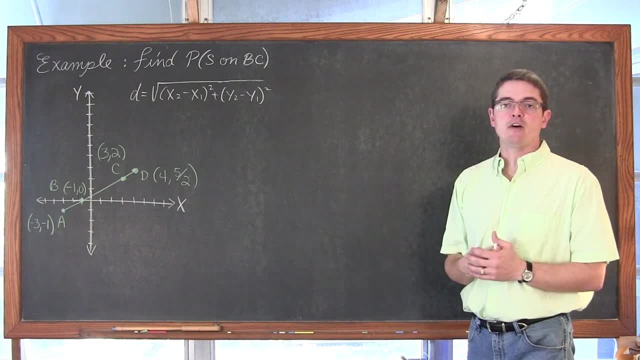 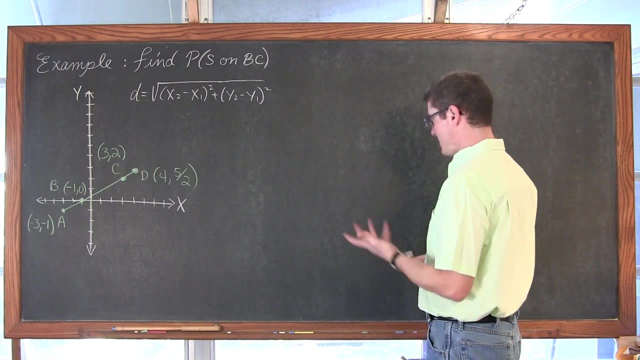 partial length, put that over the entire length And simplify it from there. So I want to find the length of BC. Well, if I'm going to do that, and let's go ahead and color code this, we're going to let this be. 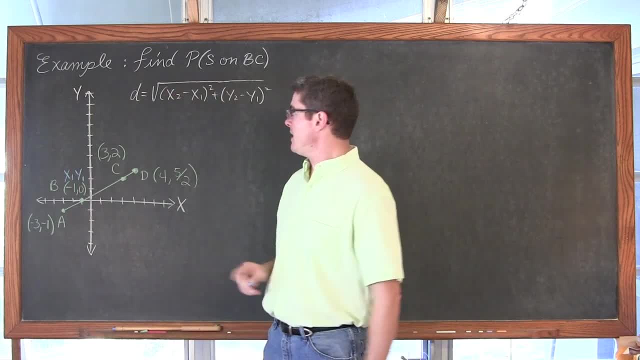 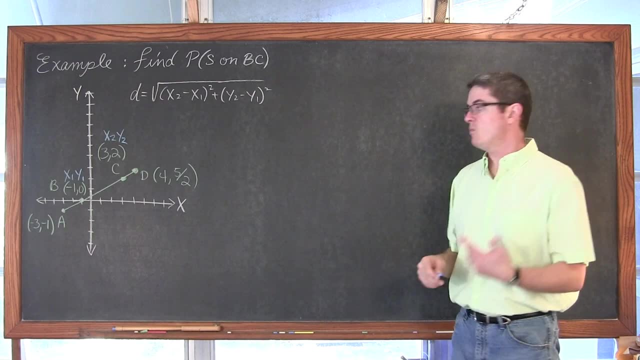 We're going to let B act as point 1 and C act as point 2.. It's a very, very good idea to make sure you've identified what you want to be point 1 and point 2 before you do anything like midpoint or slope or the distance formula, because 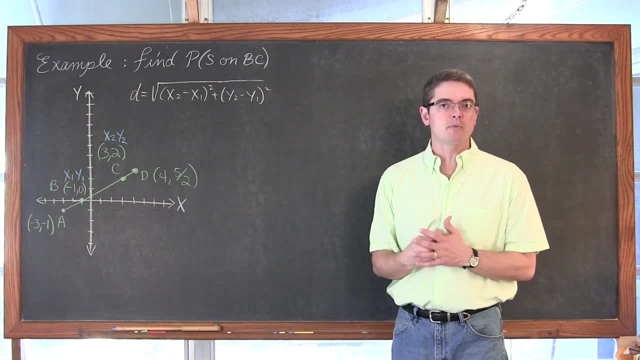 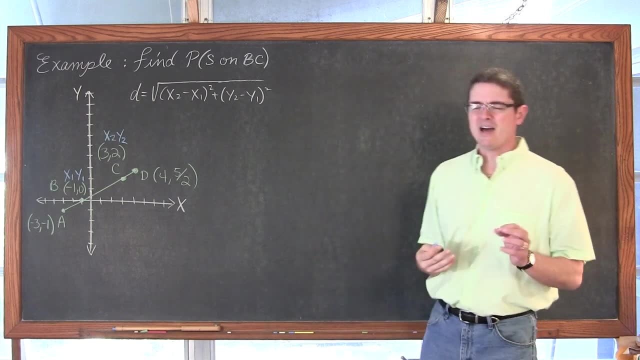 sometimes the order really Well, kind of technically It always makes a difference. but with some of those formulas if you get the order wrong as you substitute these values into your equations, you can really get the wrong answer, even though you kind of almost did it right. 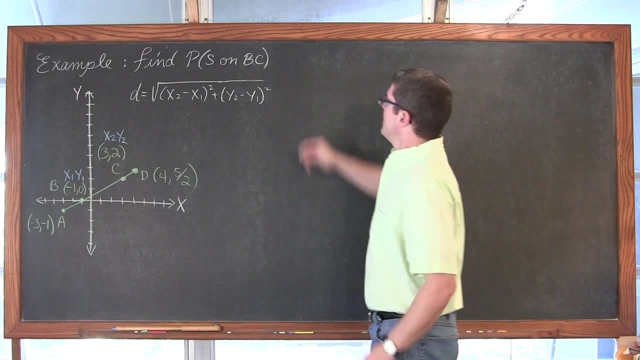 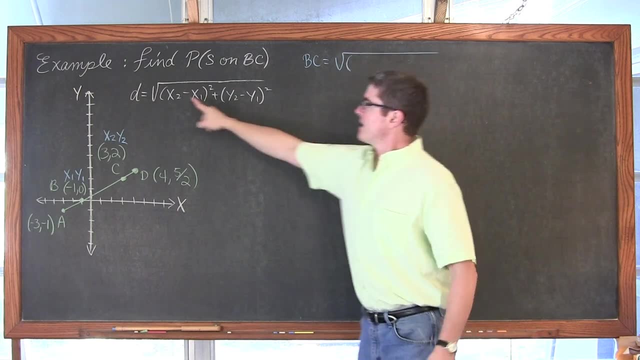 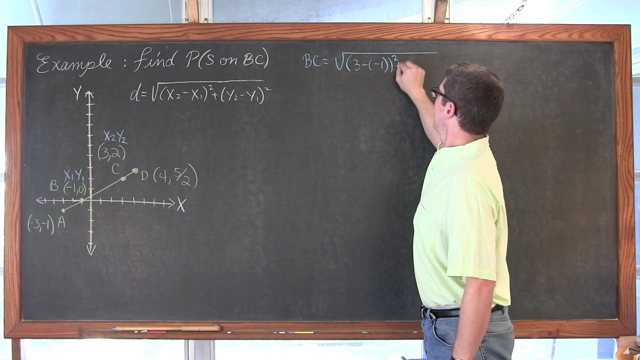 So we're going to find the length of BC again and we'll keep it in blue. So BC is going to be equal to the square root of x sub 2 minus x sub 1, so it's going to be 3 minus negative 1 squared plus y2.. 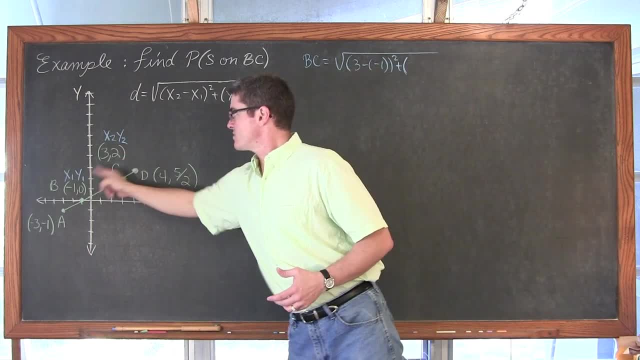 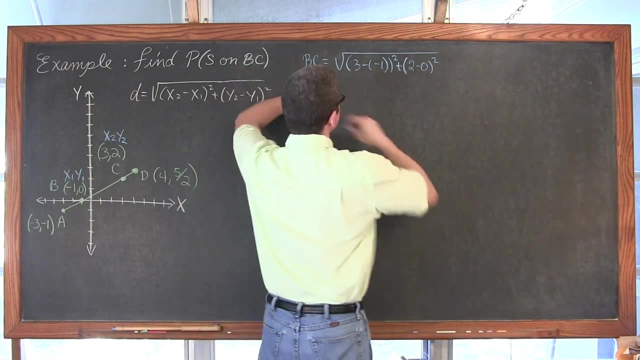 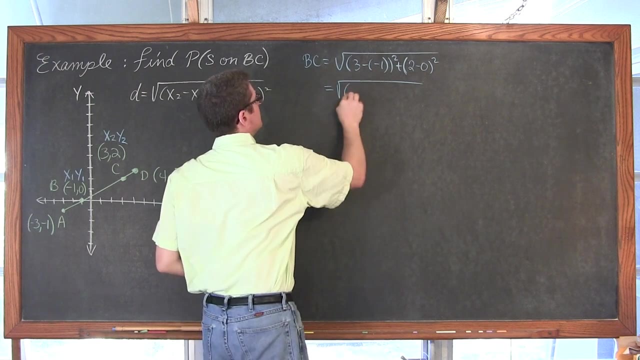 Okay, So y2 minus y1, so it's going to be 2 minus 0.. We're going to clean this up and we get the square root of That's going to be 3 plus 1, which is 4.. 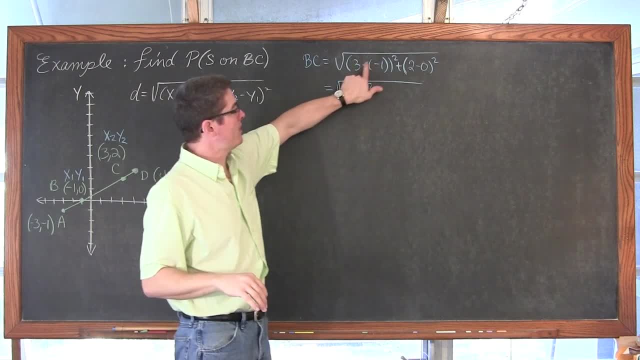 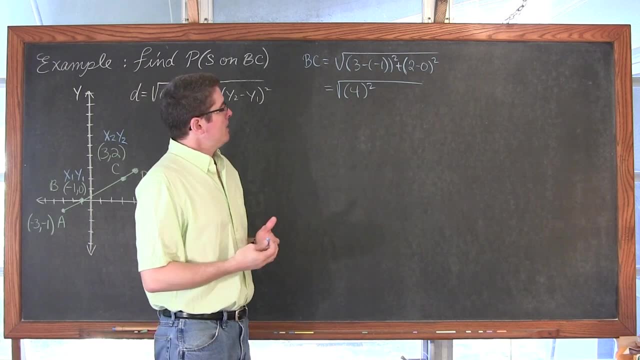 Make sure, again, you keep that wrapped in parentheses until you actually square each of these parts, because if you happen to get a negative number, which is possible as you work out the distance formula, Like Okay, Like if I had done it in the other direction, I would have done negative 1 minus 3, and 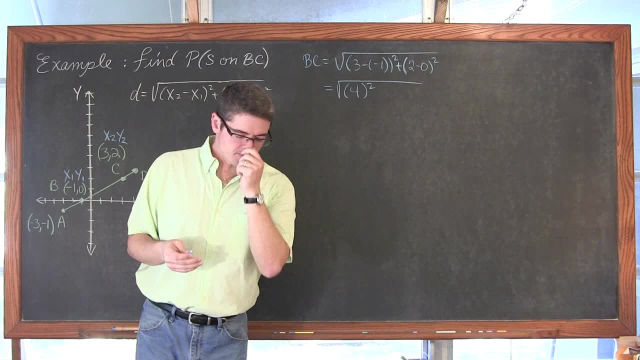 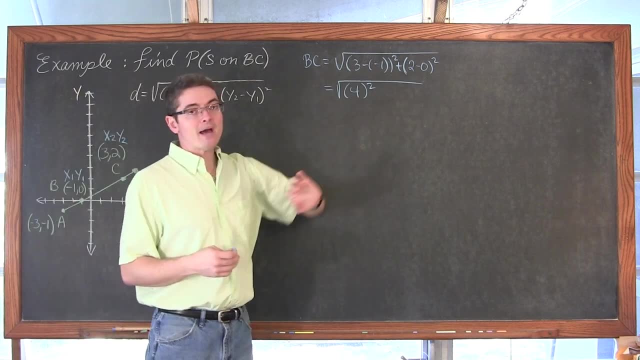 this would have been negative. 4. If you don't keep those parentheses in there, especially if you're using calculators with the two line output or the graphing calculators that you know it really matters if you get the syntax the way you have them written correct or you know they make sure that. 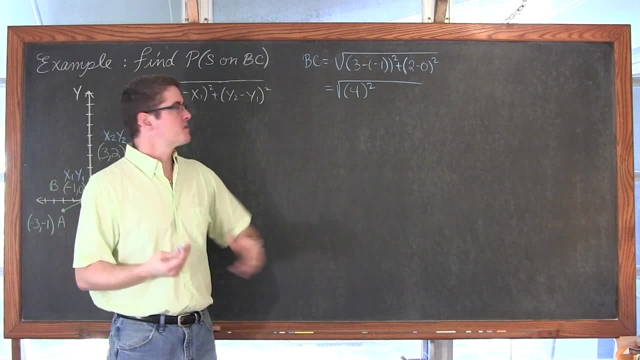 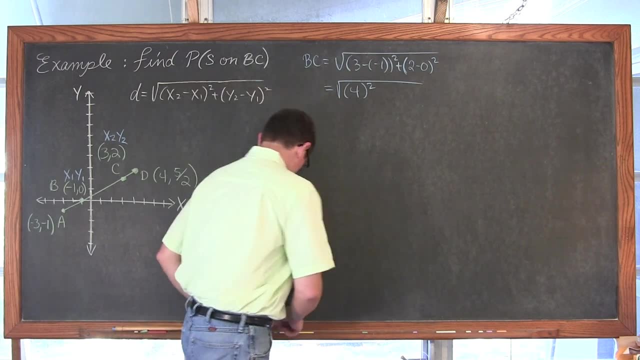 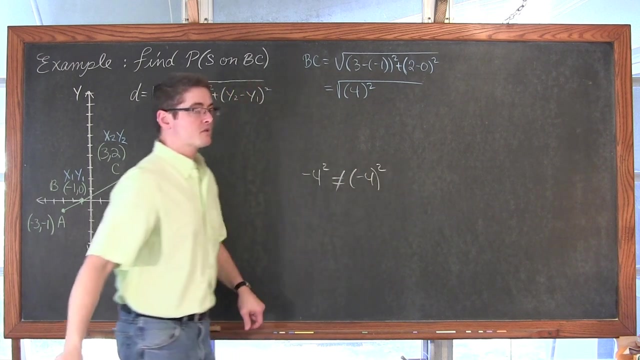 you have them written correctly. They do exactly what you type in. If your syntax is wrong and if you forget these parentheses, you will get the wrong answer. So what you need to understand is basically this: Negative 4 squared is not equal to negative 4 squared. 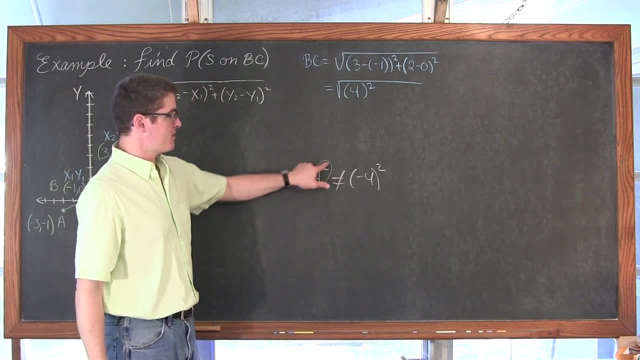 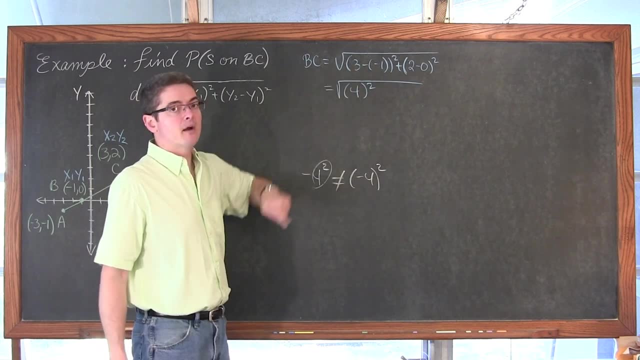 This comes out to be negative 16, because it's only the 4 that's being squared, so it's negative 4 times 4 is 16, and this with the parentheses- and they should be kept there- would come out to be positive 16, because it's negative 4 times negative 4.. 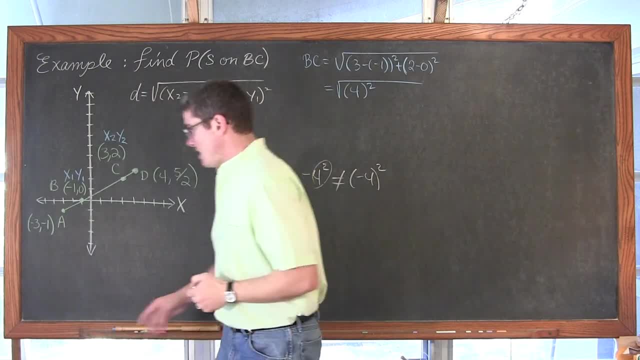 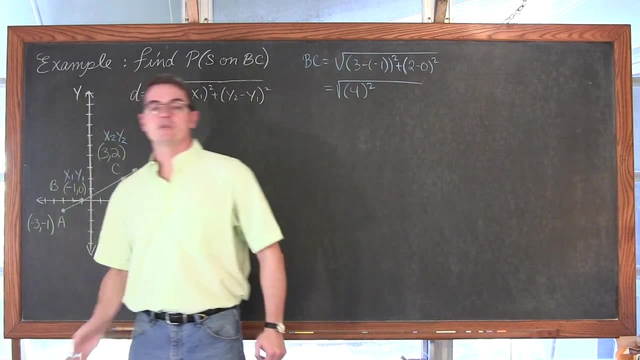 Exponents only act on what they're touching. So again, keep those parentheses in your data, Keep them in your distance formula, until you've either done it mentally, which is really the better idea, or you use your calculator so you don't get the wrong answer. 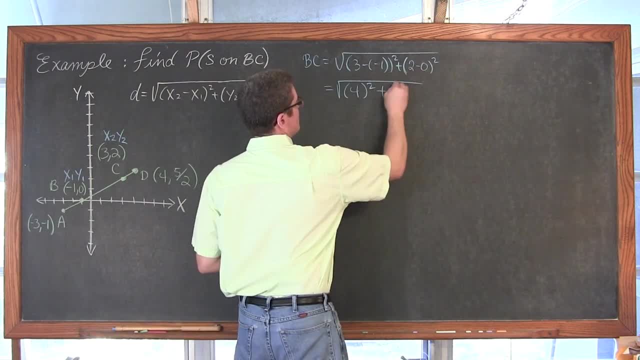 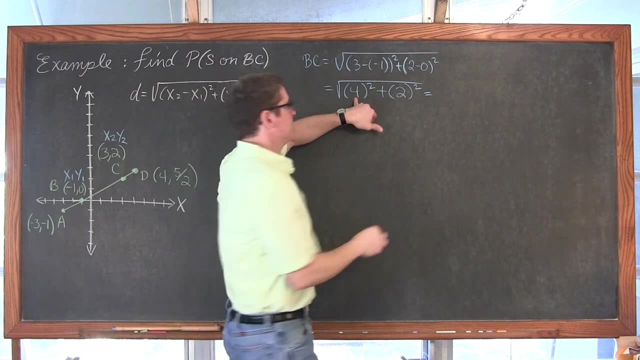 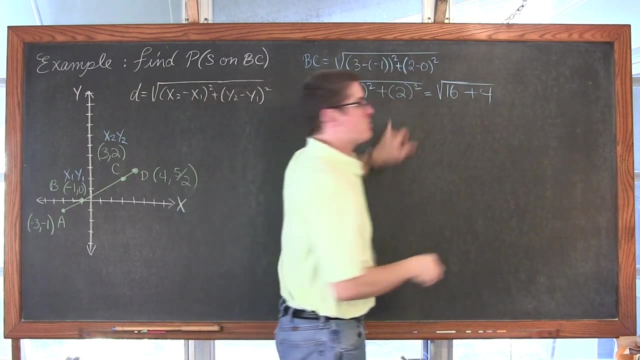 Over here we have plus 2. minus 0 is 2 squared. That means that we have the square root here of 16 plus 4.. That comes out to be the square root of 20.. And again, I like to do my videos like this: 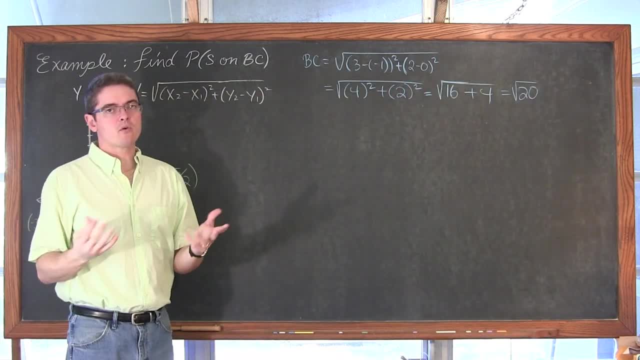 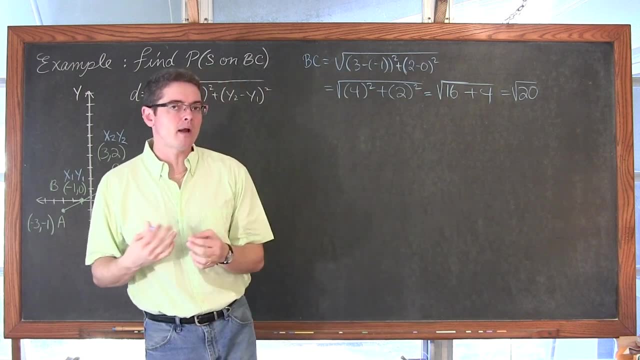 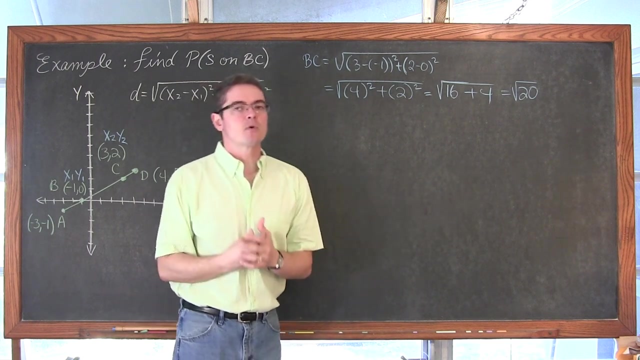 I like to do my videos in exact format because calculators, while they're great, are relied on way too often. This can be reduced. This can be reduced if there is a perfect square in 20.. Perfect squares like 2 squared is 4, 3 squared is 9,, 4 squared is 16, 5 squared is 25.. 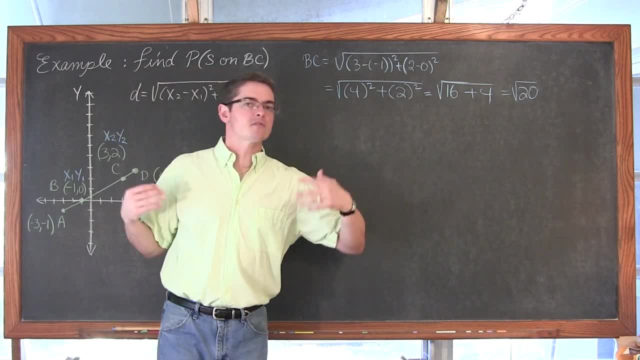 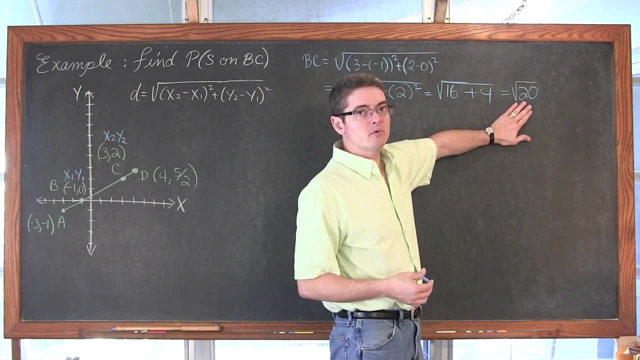 So 4,, 9,, 16,, 25,, 36,, 7 squared is 49. Your perfect squares that you can square root and get an even number. If there's a perfect square in 20, this will be reduced. 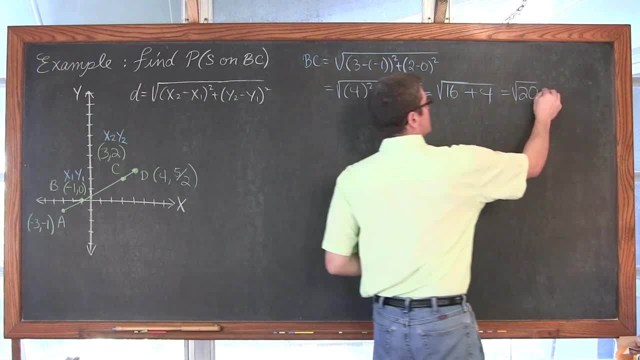 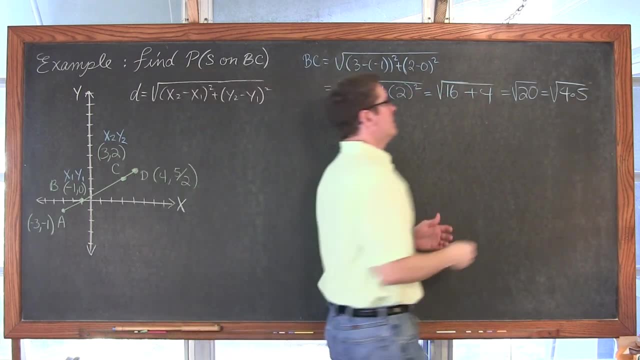 It's possible, And there is. 20 is equal to the square root of 4 times 5, and 4 is a perfect square. The square root of 4 is 2.. So our final answer is 2 squared to 5, and that is our final answer, again for the length. 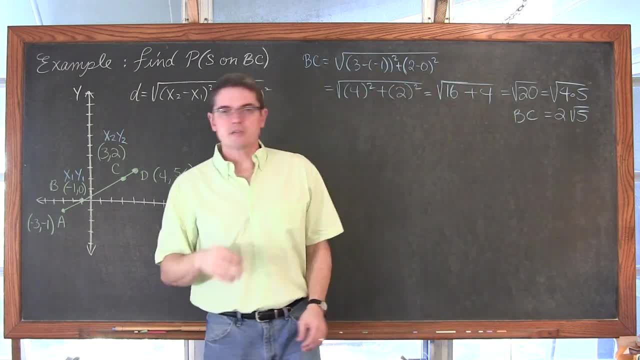 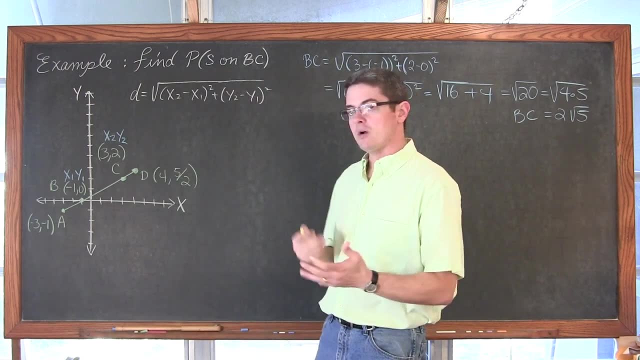 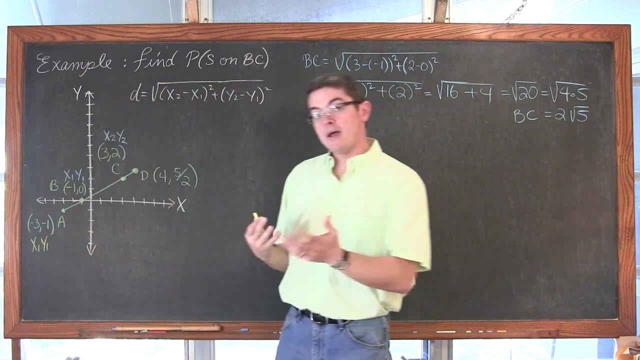 of BC. Ok, Now let's pick a different color here. I'll use yellow And find the entire length of our segment that we're working with And that is AD. Now we're going to do that. Ok, So let's call this point 1 and point, or x sub 1 and y sub 1, point 1.. 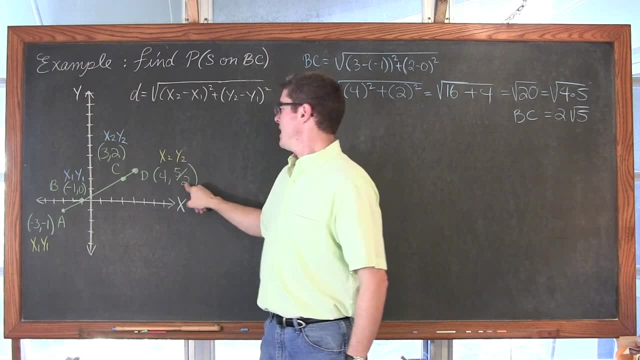 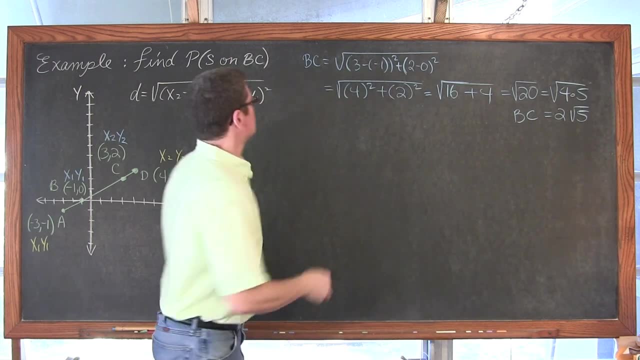 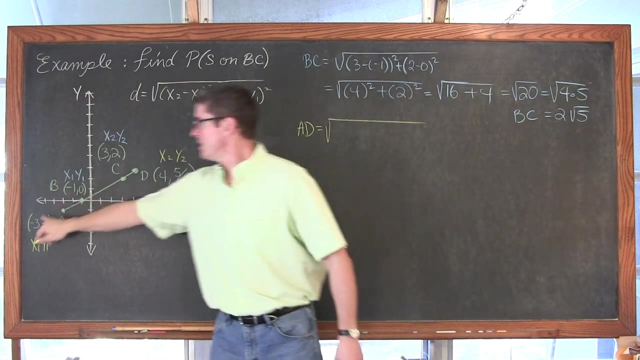 And this point 2.. Yeah, I'm going to force you to work with a little bit of algebra or fractions here to strengthen your skills, I hope. And we're going to find the length of AD. So AD is the square root of x sub 2 minus x sub 1.. 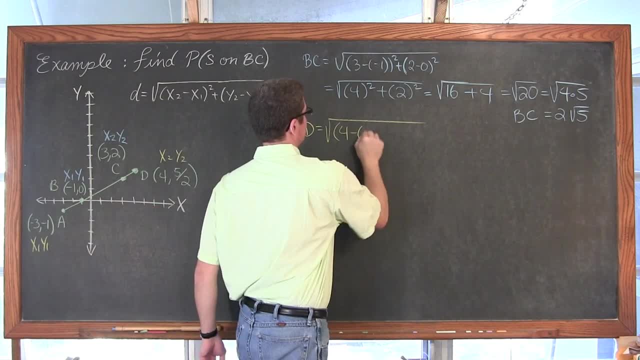 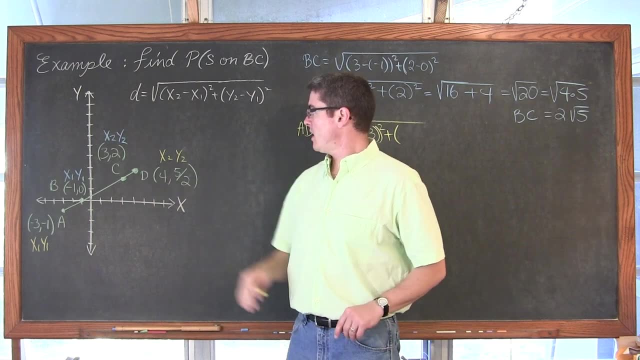 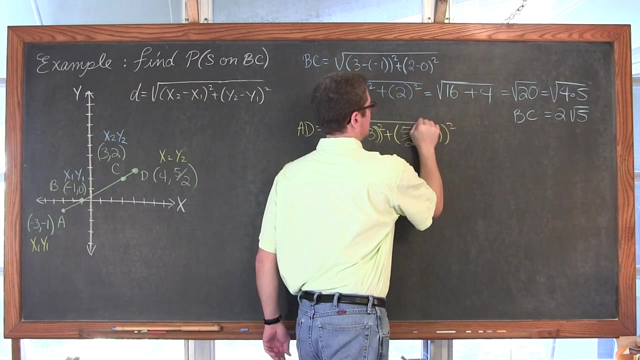 So it's going to be 4 minus negative 3.. I almost forgot my parenthesis error- Plus y2 minus y1, so it's going to be 5 over 2 minus negative 1.. And again, without being completely calculator dependent, this is going to be the square. 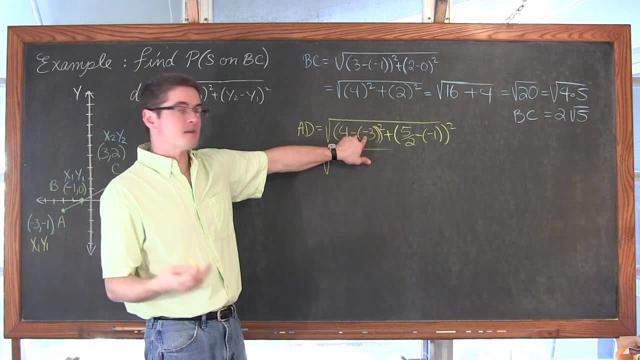 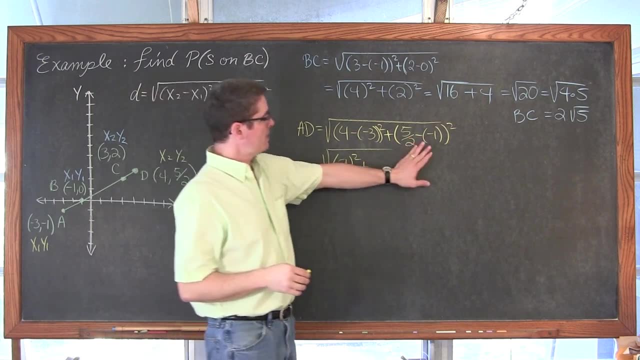 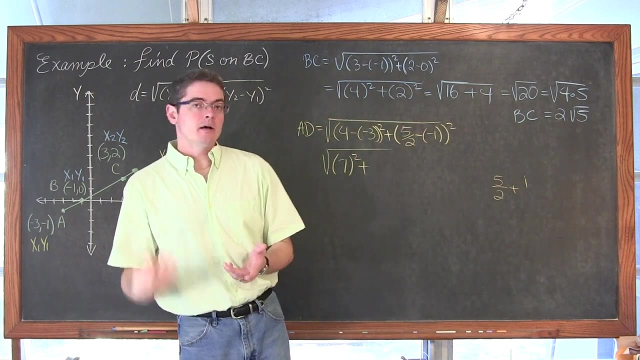 root of the two negatives. cancel out and make a positive. So 4 plus 3 is 7. And we're going to have a little bit of work over here. We have 5 over 2 plus 1.. Well, you can't add when you have fractions unless you have a common denominator. 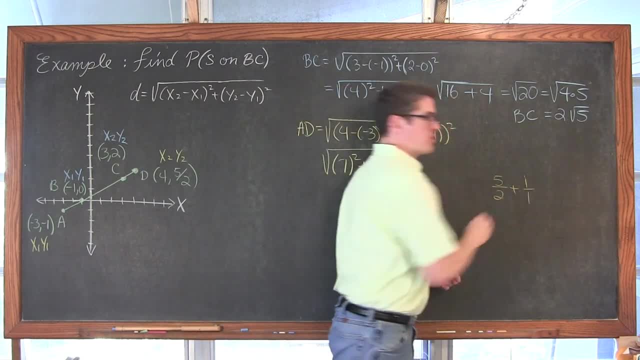 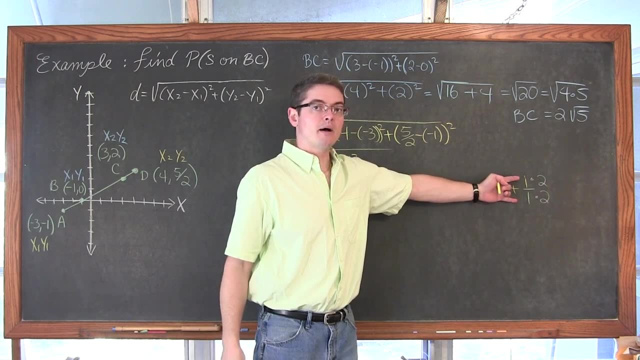 So I'm going to go ahead and write that 1, as you know, showing its denominator of 1.. I need a common denominator to add or subtract fractions, so I'm going to multiply that second term by 2 over 2, and we do that because 2 divided by 2 is 1.. 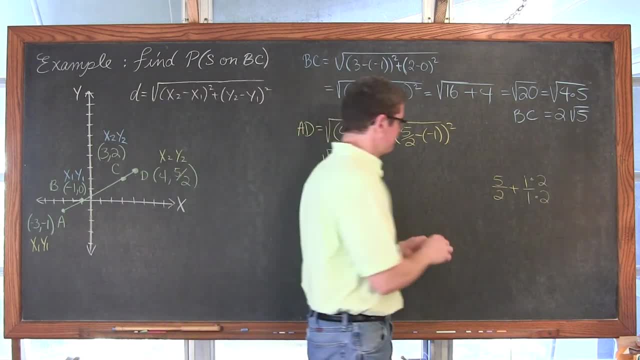 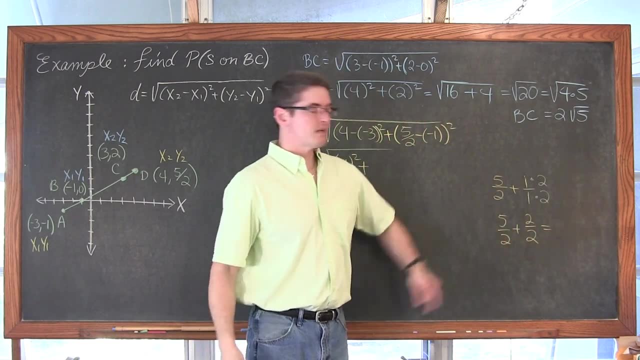 So I'm multiplying by 1, really, but I'm going to change the way the fraction looks, Ok. Ok, And now that I have my common denominators, I'm just going to add the numerators and I get 5 plus 2 is 7 over 2.. 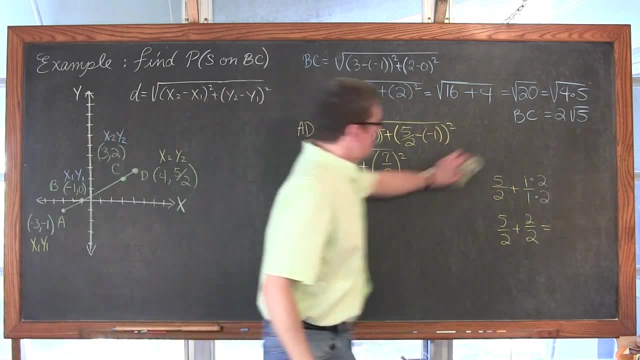 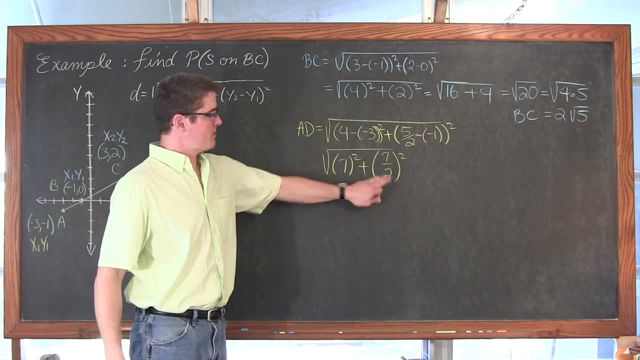 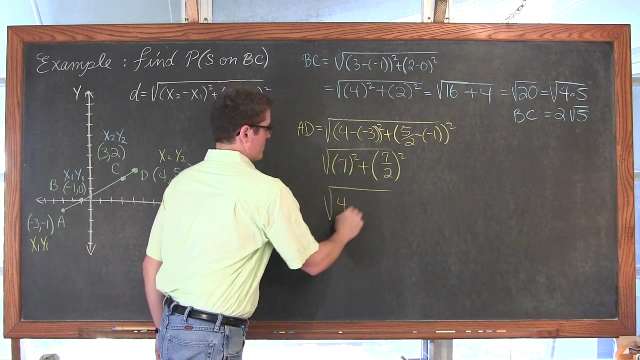 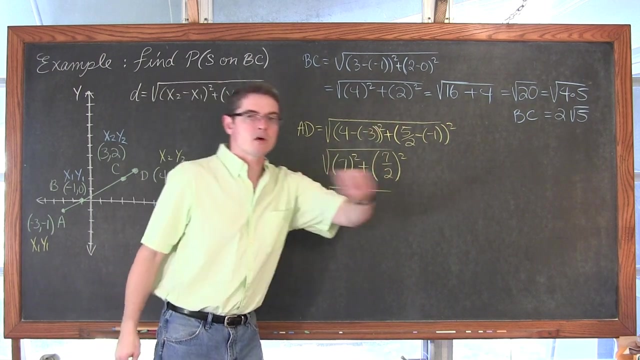 Ok, So we got. excuse me, we got to square these terms before we try and add them, which means again more practice with our fractions. So we have: the square root of 7 squared is 49.. Ok, Plus. Well, when you multiply fractions, you multiply across the top, the numerators and across 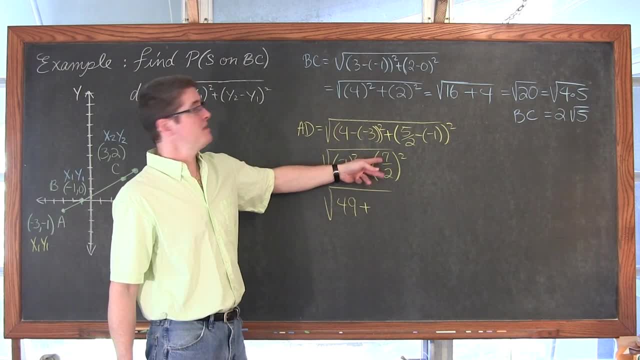 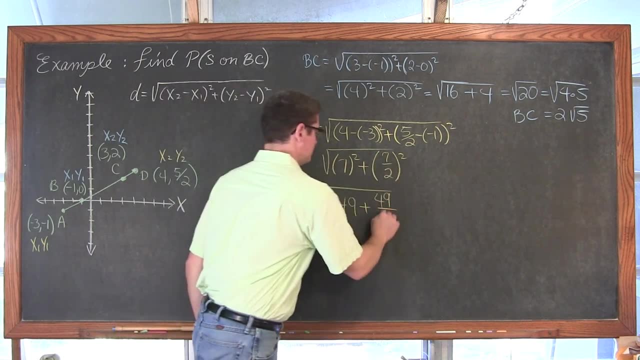 the denominators. So if you need the extra practice, just write that twice and do 7 times 7, or 7 squared is 49.. And 2 squared is equal to 4.. Ok, Well, got to now simplify this. 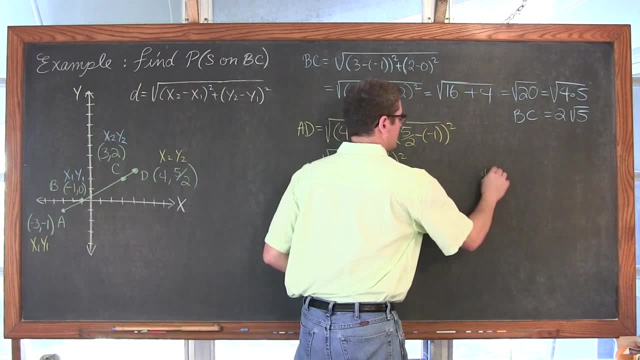 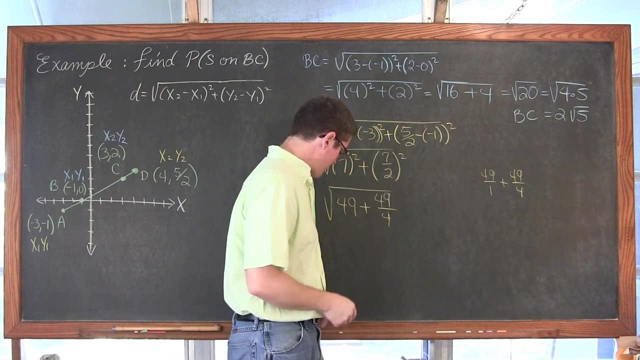 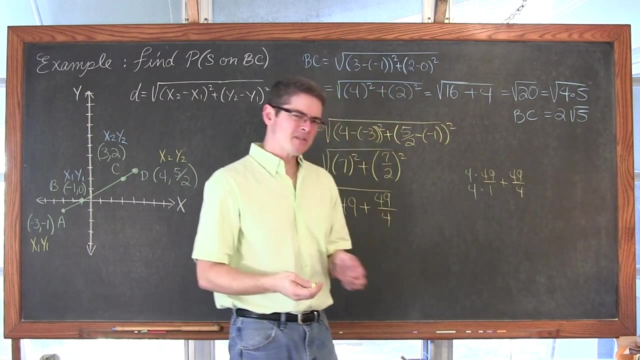 49 is over 1.. So 49 over 1 plus 49 over 4.. Ok, I need to get a common denominator, so I'm going to multiply that numerator and denominator by 4.. And now it might be a little bit difficult to do 4 times 49.. 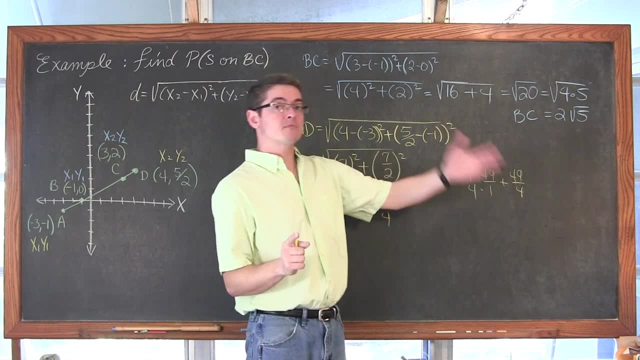 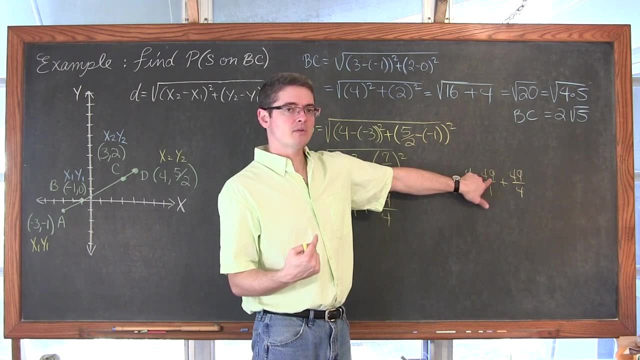 You could do 4 times 50,, which is just 1 bigger, so then you could subtract 4.. So 4 times 50 is 200, but it wasn't really 50,, it was 1 less than 49.. 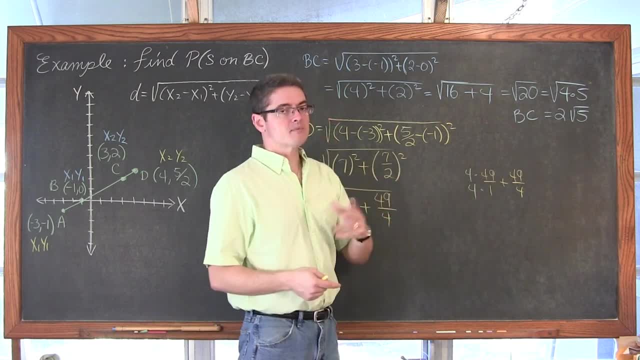 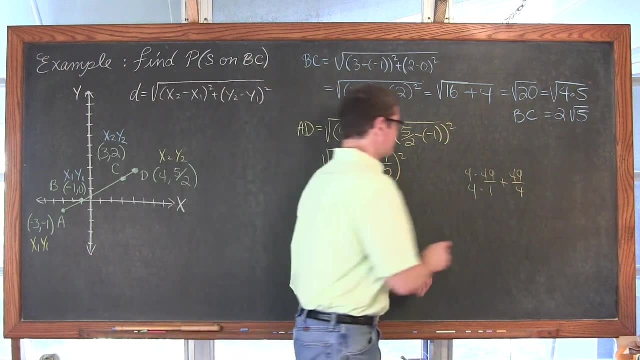 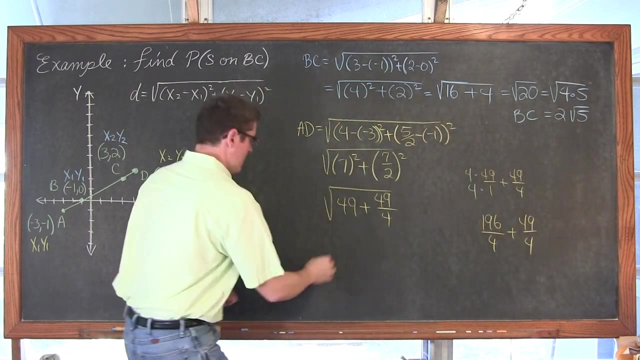 So we added that 1 extra at 50, 4 extra times, So 200.. 4 times 50 is 200, minus 4 is 196. And that is going to come out to well, let's see 190,. I'm going to drop the sixes for. 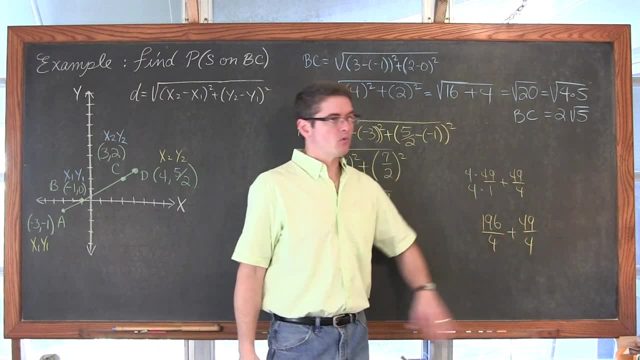 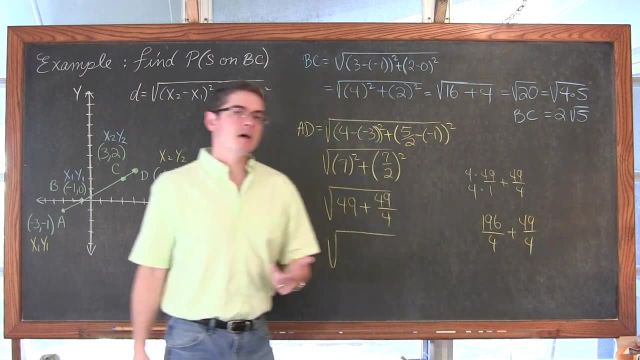 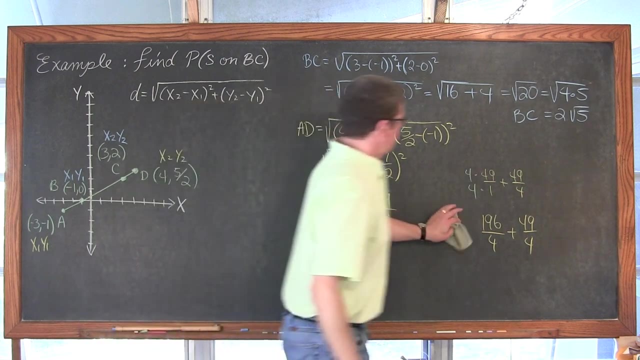 a second: 190 plus 40, 190 and 40 is 230.. Now we have 236, 236 plus 9 is 245.. Ok, I mean, you know if I'm going to guide you through a problem, I'm going to do something. 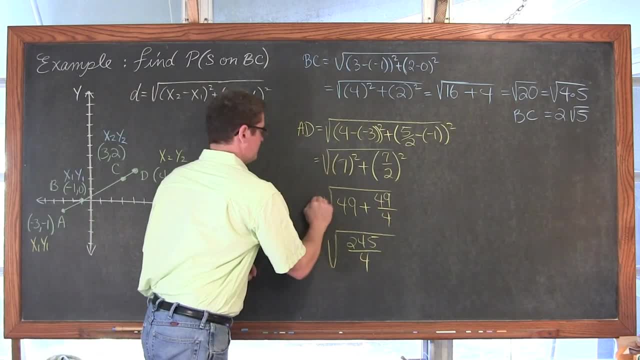 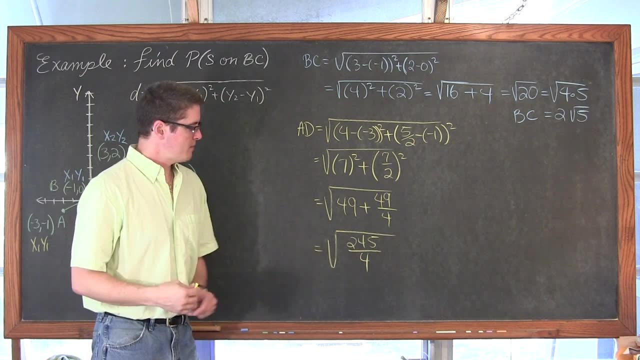 that requires a lot of math and give you some good review, right? So not everything is just whole numbers and we can't always have a calculator and use interdecimal. So this is reducible. Clearly, 4 is a perfect square, so the denominator is going to be equal to 2.. 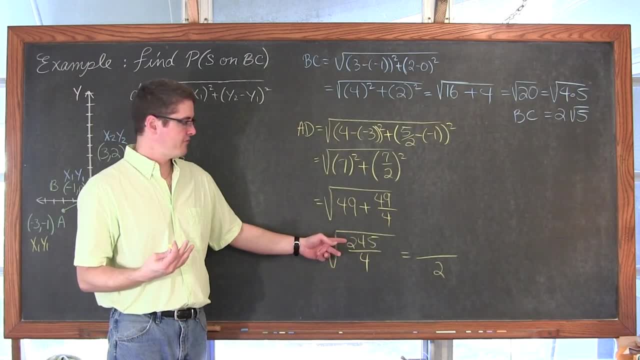 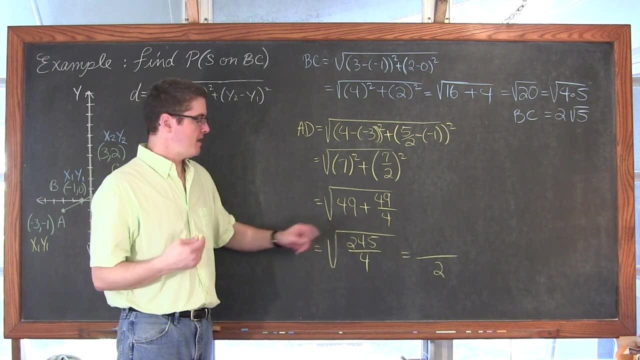 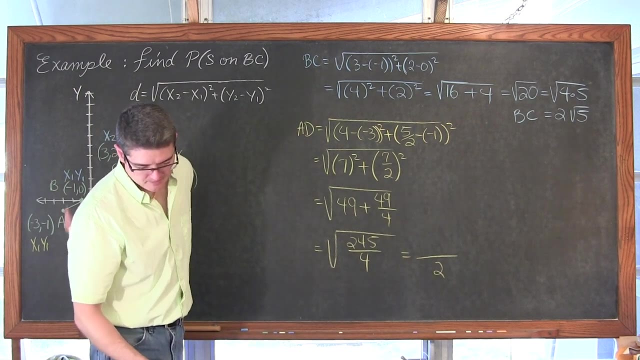 And is there a perfect square in 245?? Can I divide this by 4?? Can I divide it by 9?? Can I divide it by 16 or 25 or 36, and so on? I'm going to kind of cheat a little bit just to speed this up a little. 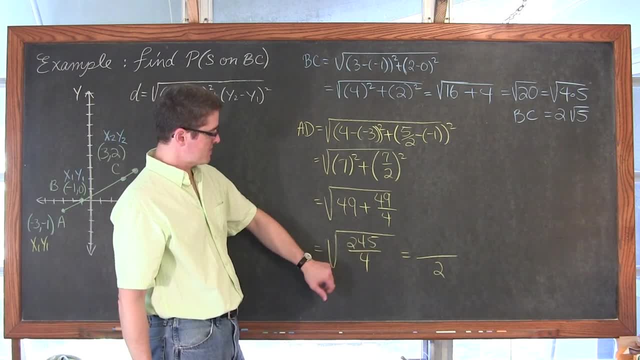 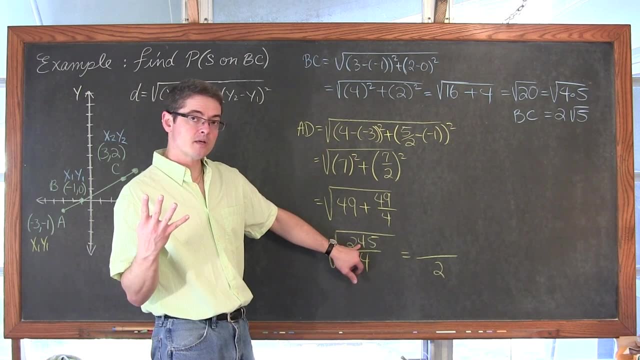 245 has a factor of 5 because it ends in 5.. So let's see here: 245 divided by 5, well, how many 5's are in 24?? 4, right, Because 4 times 5 is 20.. 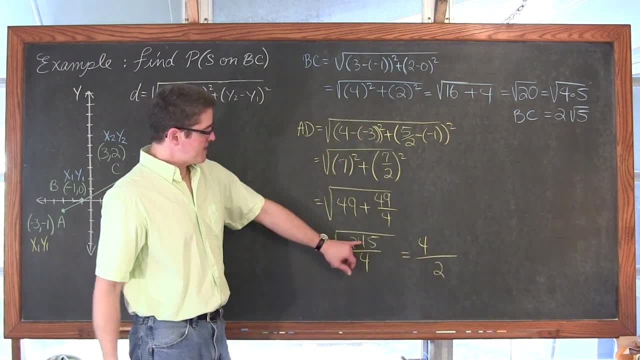 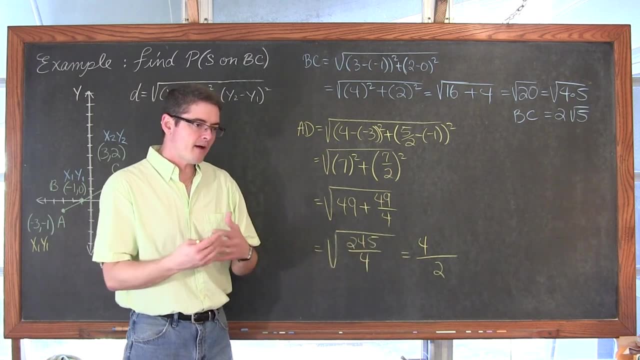 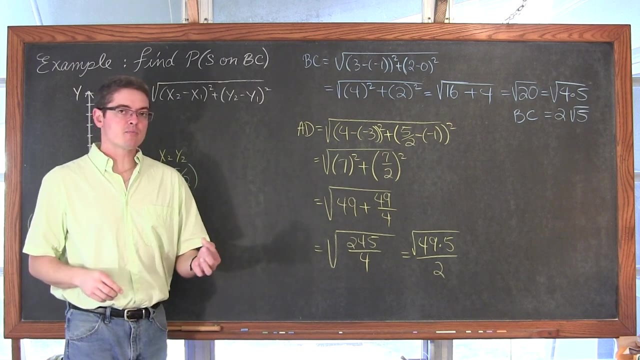 Ok. Well, if I take the 20 out of 24, that leaves me with 4,, 5, 45,. I'm dividing by 5, 45 divided by 5 is 9.. Ok, So 49 is a perfect square. so I'm reducing this radical here on top and the square root. 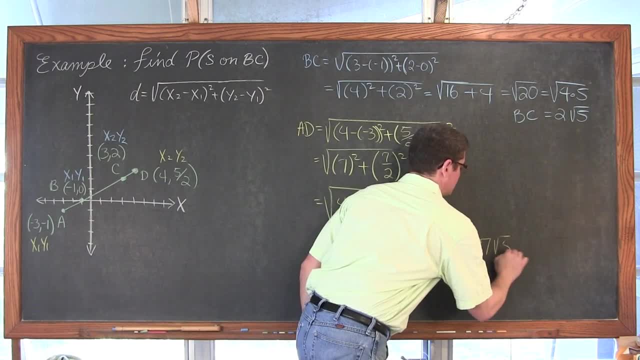 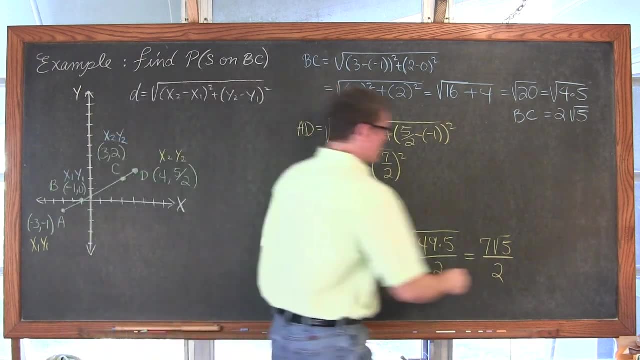 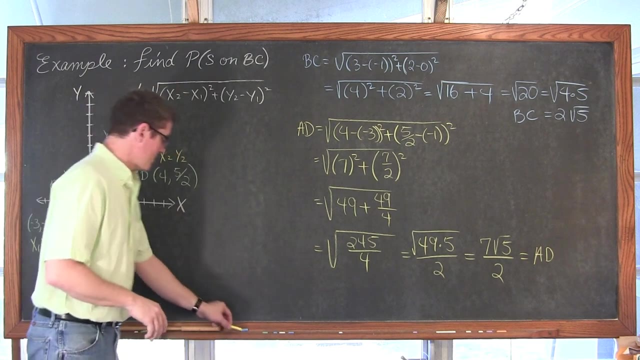 of 49 is equal to 7.. Ok, excellent, let me check my work. Good, So we have the length of BC, we have the length of AD and I think I can squeeze this in here. Let's find our final answer. 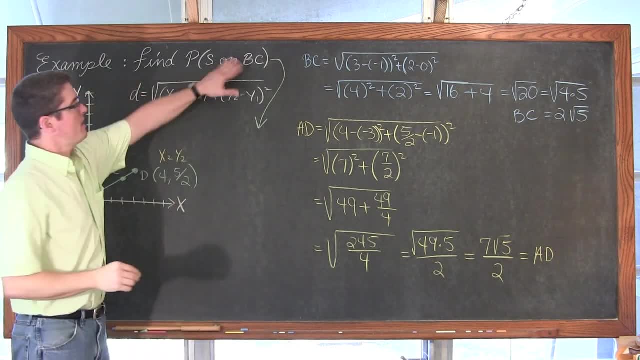 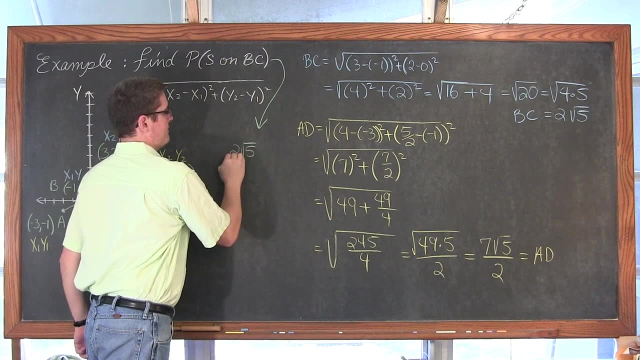 The probability that S is on BC is part over whole. the part length is 2 over, excuse me- 2 square root of 5, that is, over the entire length of 7 square root of 5, over 2.. Hmm, 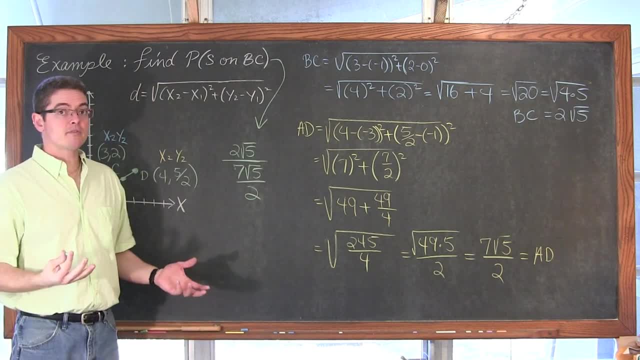 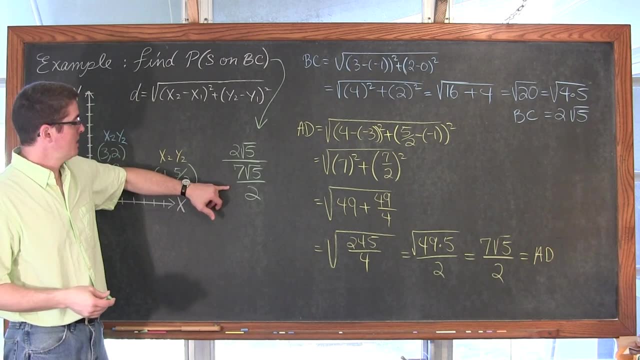 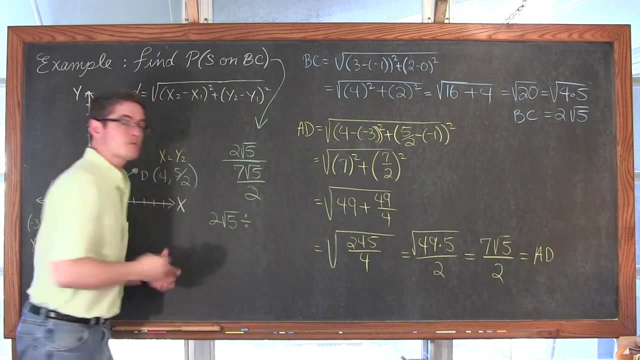 Ok, I mean, this would be a lot easier if I was just using decimals for my calculator. Let's see how long has it been since you have divided by a fraction 2 over 5, I keep saying over 2, square root of 5 divided by, because that's what a fraction. 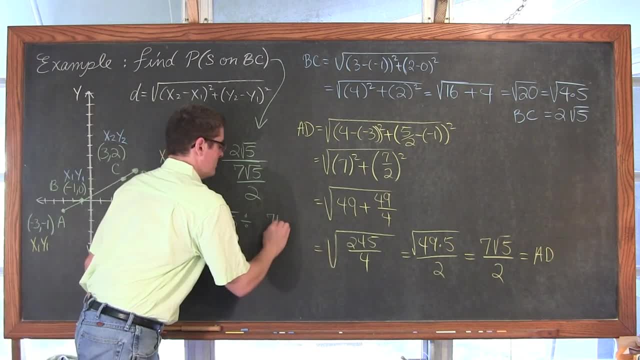 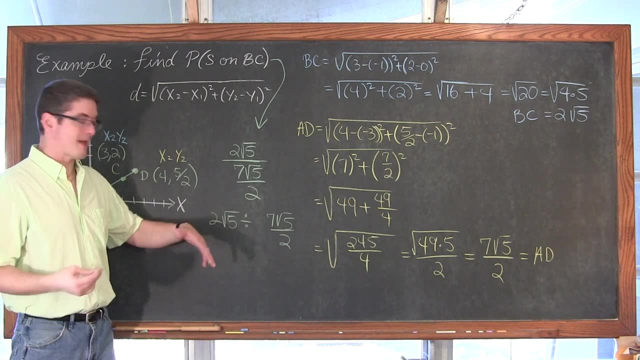 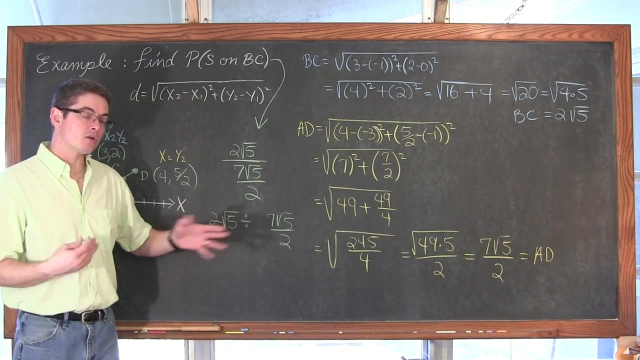 bar means 7 square root of 5 over 2.. You really can't divide fractions. you can only multiply by the reciprocal of the second fraction, or that is how you divide fractions. So I'm going to also make both of these factors look like a fraction, so I make sure they. 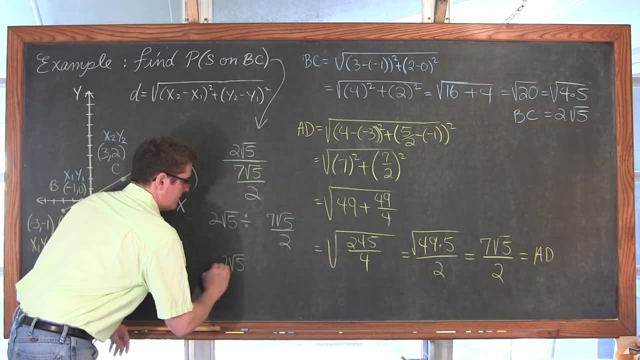 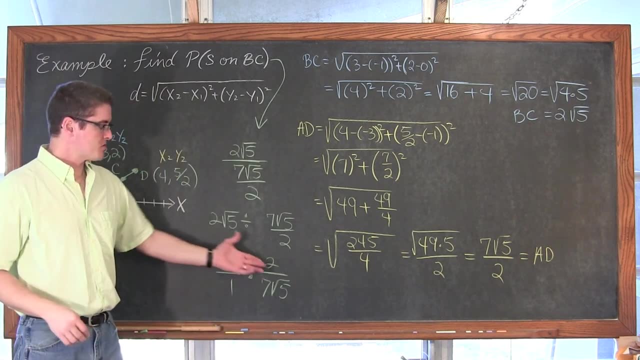 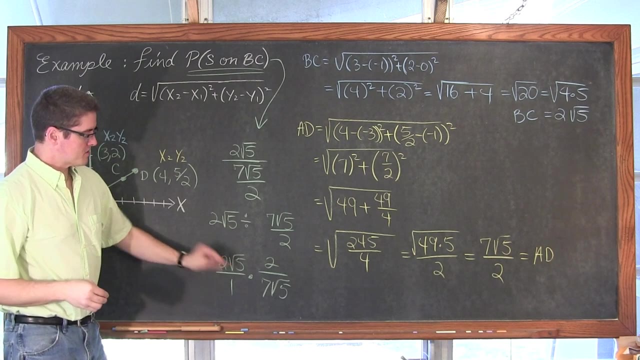 get them lined up properly, We're going to have 2 square root of 5 over 1 times 2 over 7 square root of 5.. And all those work with those radicals. and then my final answer of the probability that S is on BC with the square root of 5 in the numerator and the square root of 5 in the. 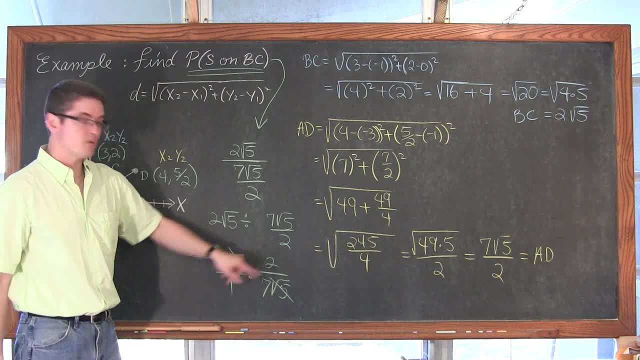 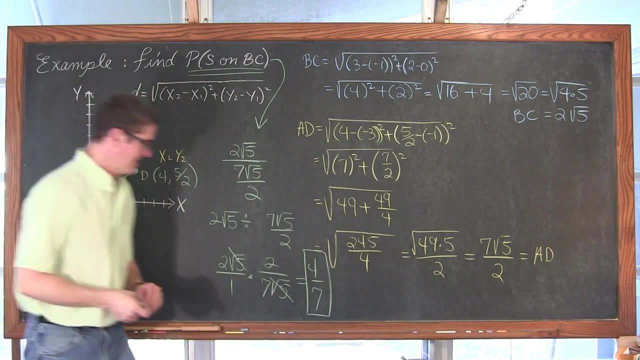 denominator. they are going to cancel out, And I just get left with 2 over 5.. 2 times 2 is 4 over 7.. That's it. It's not too bad if you remember how to- let's see- do the distance formula. make sure you. 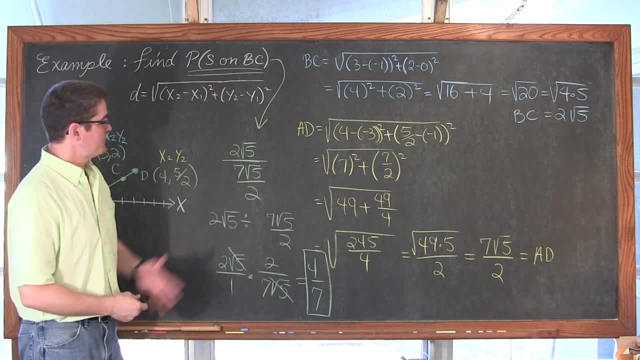 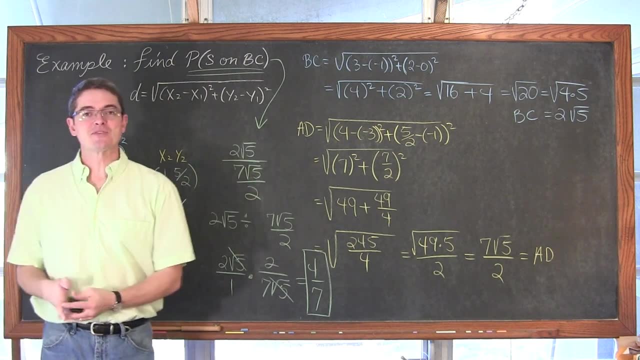 watch your signs, remember how to reduce radicals and then, finally, you know how to divide fractions, Hopefully something you can practice a lot in your math classes. but if not, there you go. I'm Mr Tarrou BAM.